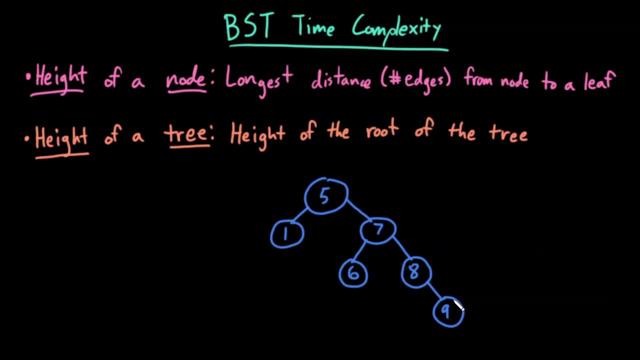 Nine is a leaf. so the distance between nine and a leaf, in terms of counting number of edges, the longest possible distance is zero. Nine is the leaf. so there are no edges between nine and a leaf because it is a leaf. So the height here: 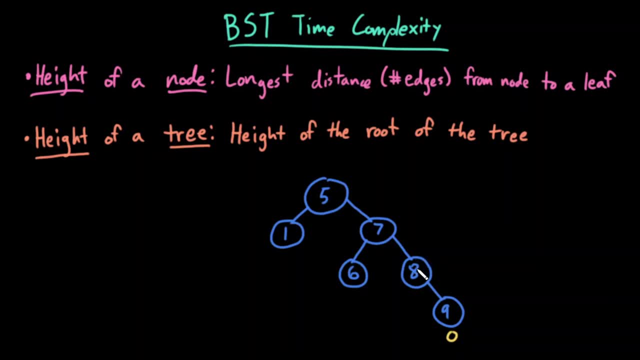 is zero. Eight. the only leaf below it is nine and the path from eight to nine has one edge. so the height of eight is one. Seven has two leaves below it, it has six and it has nine. The path from seven to six has one edge. the path from seven to nine has two edges. 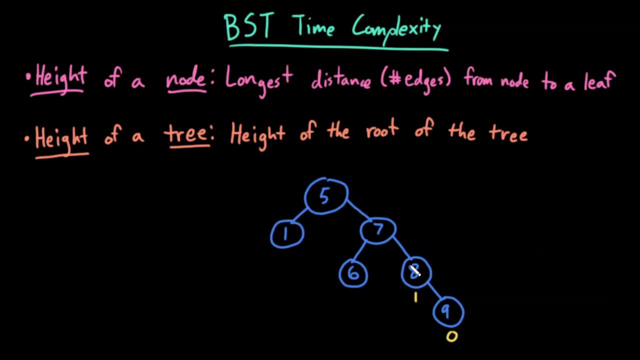 therefore the height. it's the longest of these distances, which is two. Out of all possible paths to a leaf, we take the longest one And then five has three leaves below it: one, six and nine. The path from five to one is distance one. the path from five to six is distance two. 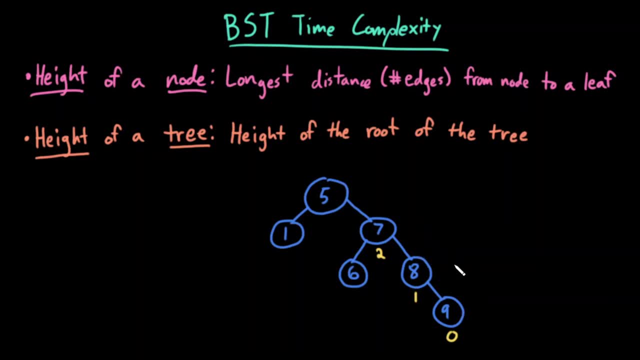 and the path from five to nine is distance. one, two, three. The largest of these is three. so the height of five is three, and then one and six are leaves. so, just like with nine, their heights are zero. If you think about this, we can actually think of a simple algorithm for computing the heights. 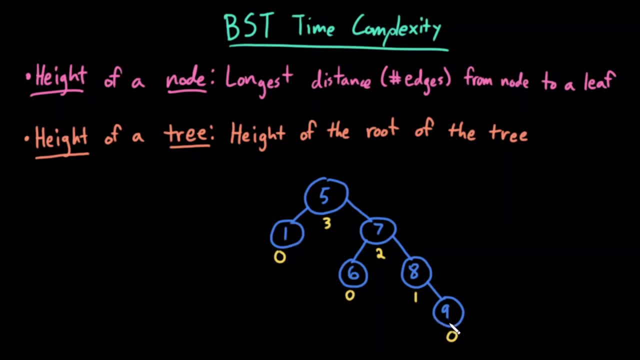 of every single node. We could theoretically do a post-order traversal where, if the current node is a leaf, its height is zero. Otherwise, if it's an internal node, its height is one plus the largest height of any of its children. So here nine is a leaf, so its height is zero. 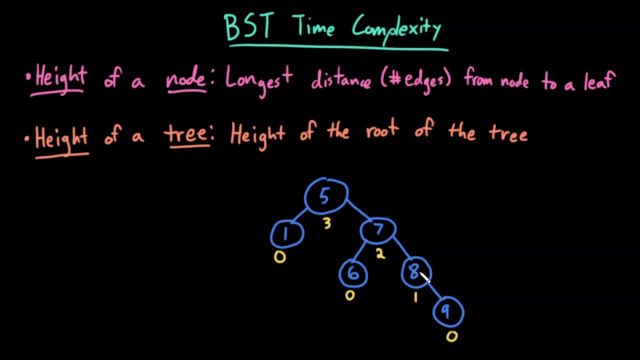 Eight is not a leaf. therefore its height is one plus the largest height of its children. Its only child has a height of zero. therefore its height is one plus zero. Six and one also have heights of zero because they're leaves. Seven is an internal node, so its height is one plus the height of its largest child's height. 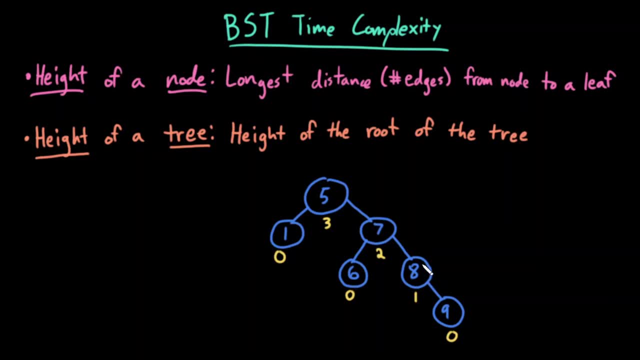 So its two children have heights zero and one, so the larger height is one, so its height is one plus one, which is two. And then, same here, its children have height zero or two. two is the bigger one, so its height is one plus two, which is three. 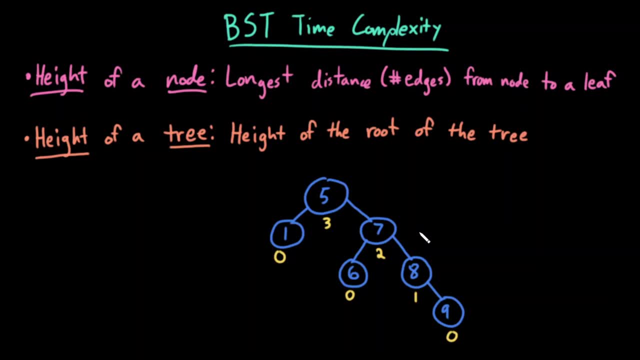 So pretty easy to do visually and it's actually a fairly simple algorithm to implement. So that's how we compute the height of the nodes in our tree. What about the height of the tree overall? We define the height of a tree to be the height of the root of that tree. So for this, 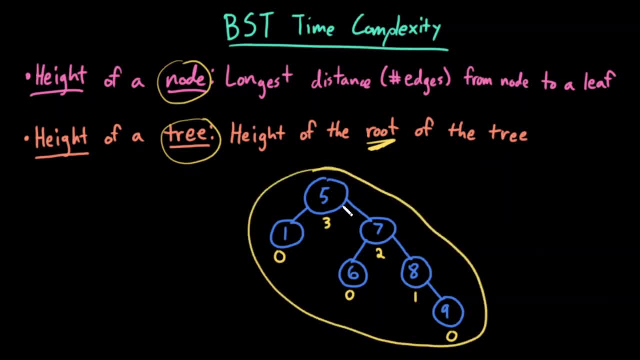 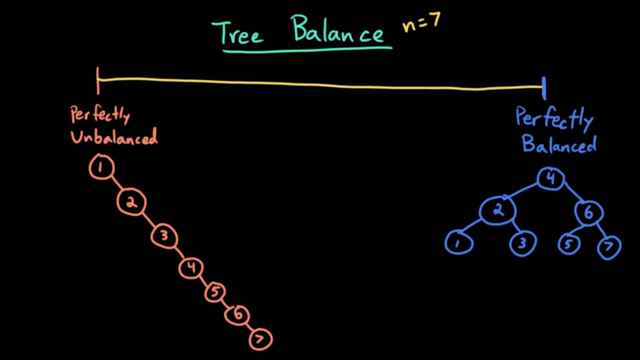 entire tree. the height of the tree is the height of the root, which is the height of the tree. So we say this tree has height three. We can start to describe time complexity with respect to tree balance. So we can think of tree balance as being this metric of how tall a tree is, with 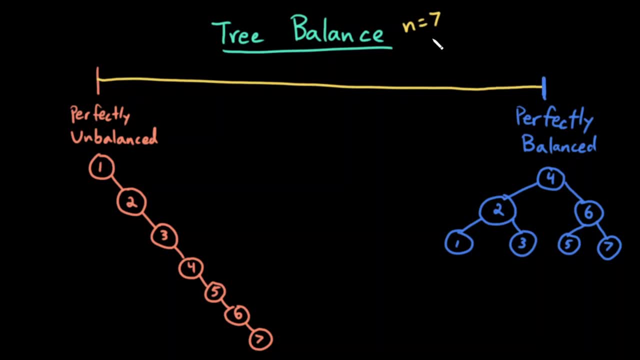 respect to the number of nodes it has And we can think of it kind of as a spectrum. So, given some n, some number of elements, number of nodes in my tree, I can think of tree balance as being a spectrum between perfectly unbalanced and perfectly unbalanced. So we can think of tree 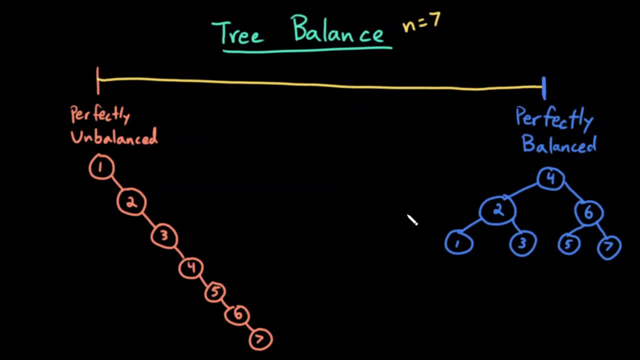 balance as being perfectly balanced. So here I have two binary search trees. Both contain the exact same elements. The number is between one and seven. But here I have a perfectly unbalanced tree where the height here- one, two, three, four, five, six- is six. So the height of this tree, 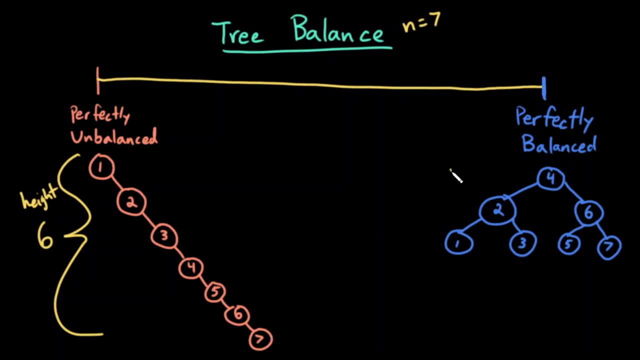 is six versus. here It's the exact same elements, also a valid binary search tree, But the height here is two. So in general, as the number of elements grows, the height of our tree must also grow. If I have more elements, I must have more edges to connect them. But a perfectly 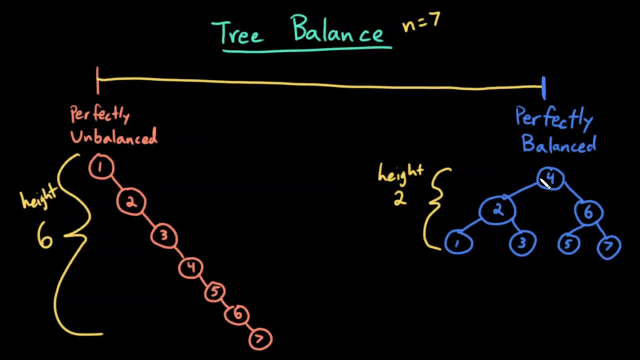 balanced tree minimizes the height of the tree with respect to number, with respect to how many elements it contains, versus a perfectly unbalanced tree maximizes the height of the tree With respect to the number of elements. So these are both binary search trees And we can think. 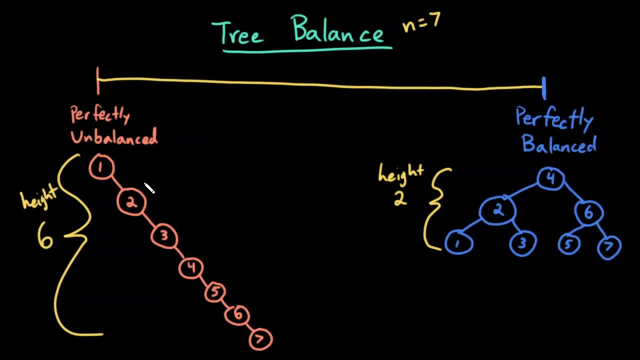 about how fast or how slow a find, insert or remove algorithm would be. So remember all three of those algorithms. the first step is performing the find operation. So that is actually the rate limiting step of all three of those algorithms. For a perfectly unbalanced tree, I have seven. 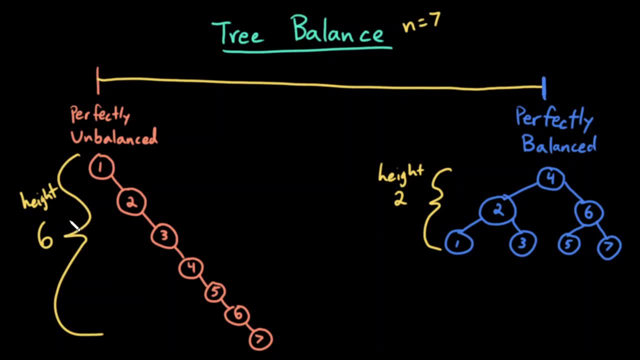 nodes and my height is six. So I have a perfectly unbalanced tree and my height is six, So I have seven minus one, which is six. So in general, if I have n nodes, n elements, a perfectly unbalanced. 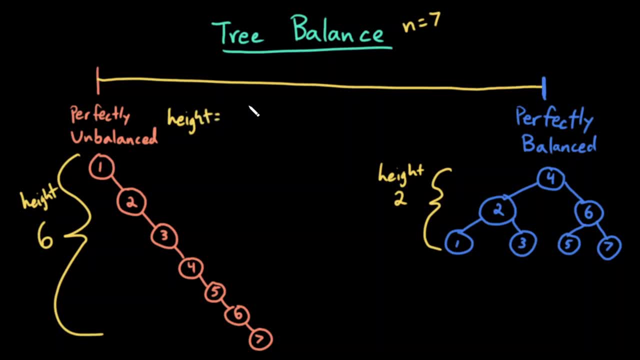 tree will have height equals n minus one. It's essentially just a linked list where I have n nodes and I have an edge connecting them in a chain. So the height would be n minus one. Therefore, the worst case- big O time complexity for find, insert or remove- would be big O of n In the worst case. 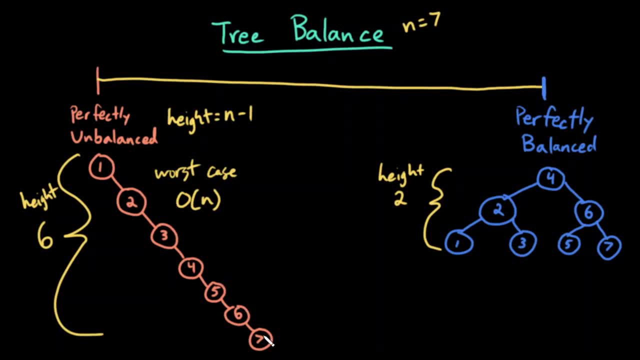 I would have to traverse over all of the edges of my tree- And I have big O of n edges- in order to find the element or find the site of insertion or find the removal site. So, for example, let's say I want to remove seven from this tree, Removing seven, I would start at the 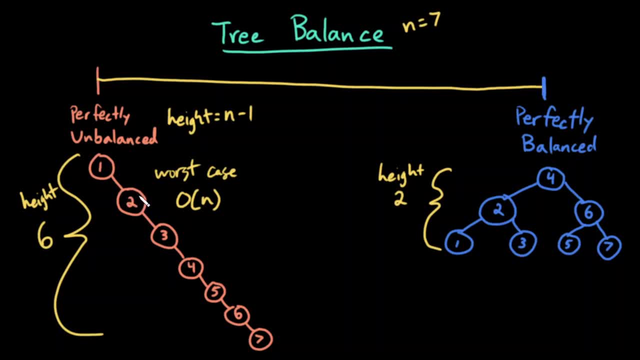 root Seven is bigger than one. traverse right Seven is bigger than two. traverse right Seven is bigger than three. traverse right Seven is bigger than four. traverse right Seven is bigger than five. traverse right Seven is bigger than six. traverse right: Oh, seven is equal to seven. 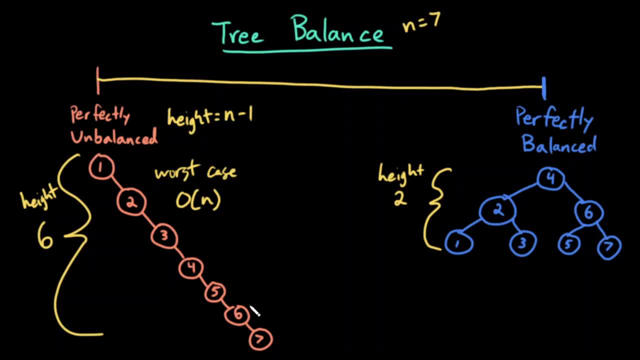 I can remove it. So for remove, I had to traverse big O of n edges. For find, I had to traverse big O of n edges. And for insert, let's say I wanted to insert eight into this tree. I would do the. 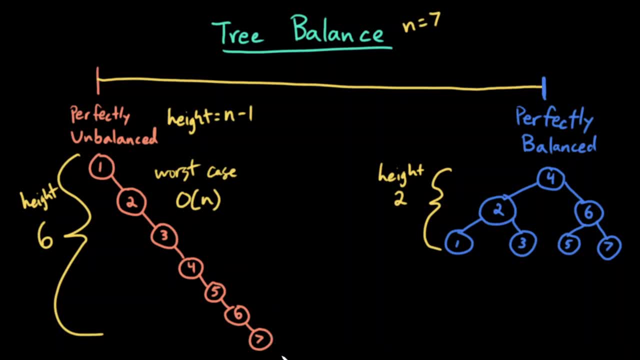 exact same big O of n find operation and then just insert here. So the worst case: in a perfectly unbalanced binary search tree, all three of my operations are big O of n In a perfectly balanced tree- my height is two- which this is actually log base two. 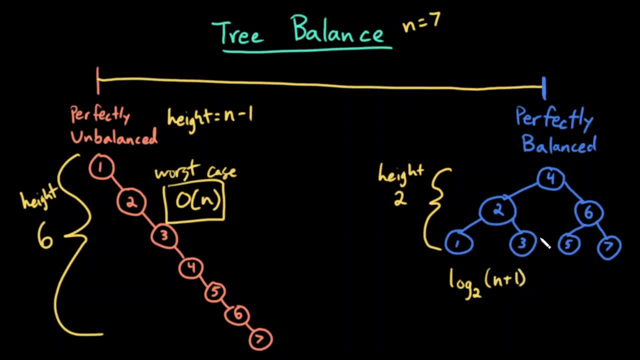 of n plus one minus one. it might be a little complicated how I just kind of pull this out of my head. Don't worry about it. Just think if I almost doubled the height of my tree, so if I added one. 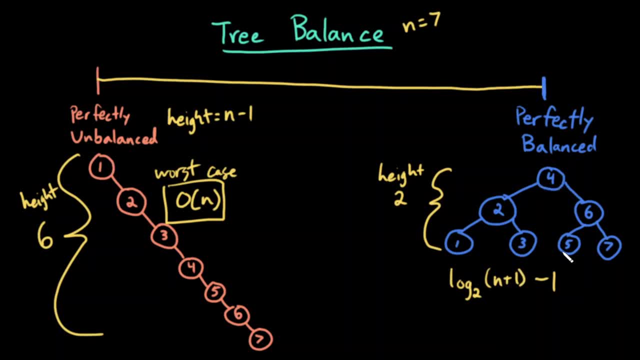 two. I mean sorry if I almost doubled the number of nodes in the height of a perfectly balanced tree, sorry if I almost doubled the number of nodes in a perfectly balanced tree. I would add one more row of one, two, three, four, five, six, seven, eight. I would add two children to each of. 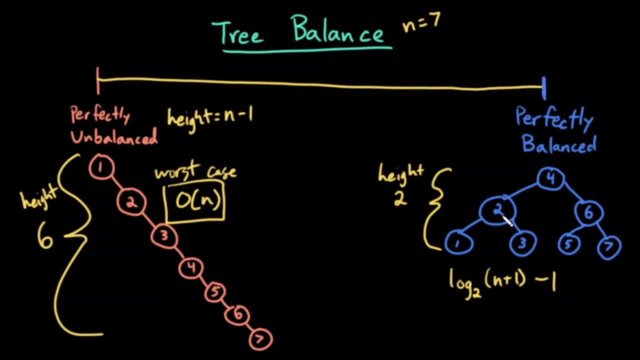 the bottom row. My tree currently has seven. I would add eight. I've essentially doubled the number of nodes in my tree, but my height would increase by one. So you can maybe think about this a bit more to see how we would derive this function. but with n equals seven nodes. it's log base two. 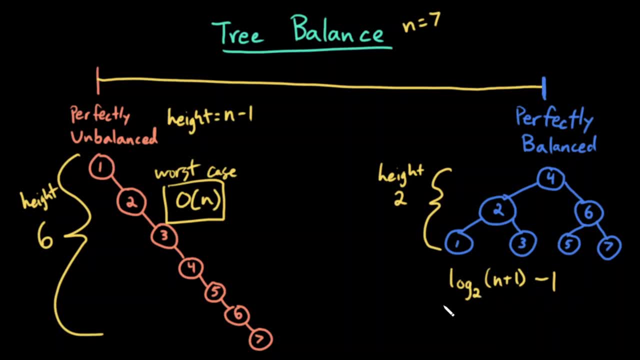 of eight, which is three, minus one, which is two, So in a perfectly balanced tree, our three operations are big O of log n right. This is the dominant term. However, this is not the worst case scenario. This is not the worst case, This is actually. 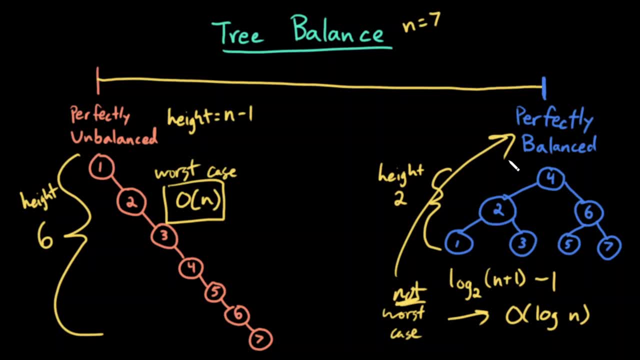 a very nice case. This is the case when my tree is perfectly balanced. So the worst case time complexity for a binary search tree in general is big O of n. If my tree was perfectly balanced, the worst case time complexity would be big O of n. 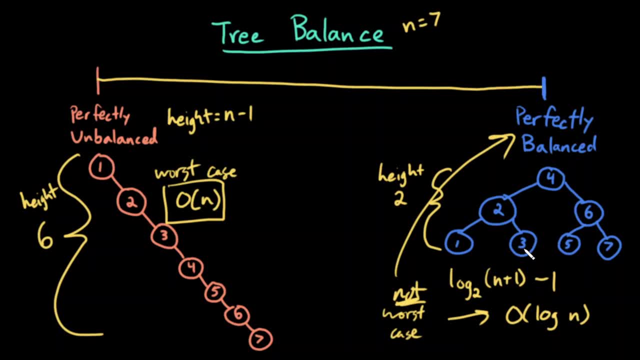 But for a just general, arbitrary binary search tree, I'm not guaranteed that it will be perfectly balanced. So for some general binary search tree, this big O of n term is what you want to remember as the worst case time complexity. In the future we will talk about other binary search tree data. 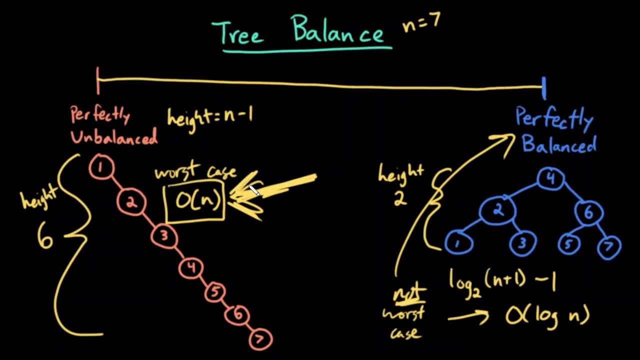 structures that are what we call self-balancing, And these self-balancing binary search trees do give us a guarantee of some notion of tree balance, But just in general for an arbitrary valid binary search tree, we have no such guarantees of height. Therefore, the worst case is big O of n. 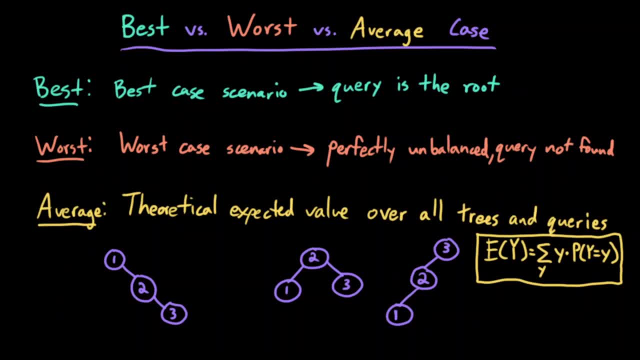 Let's talk about the best case, worst case and average case time complexities of the find algorithm of a binary search tree. In general, the best case time complexity happens in our best case scenario. Generally speaking, these are given n elements, So we have n elements where n approaches infinity. 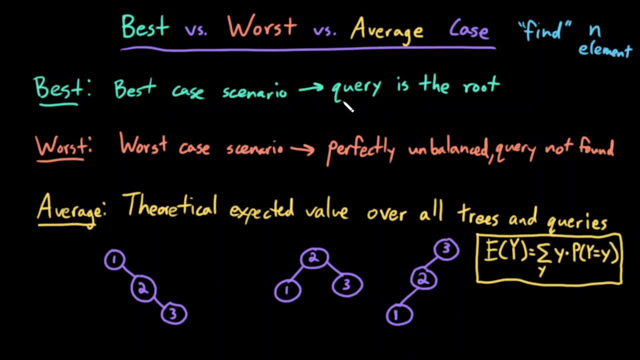 So the best case time- complexity is the best case scenario which for a binary search tree find- is when the query, what we're looking for, happens to be the root. So here, if I'm searching for node one, the first node I check is the root, which is what. 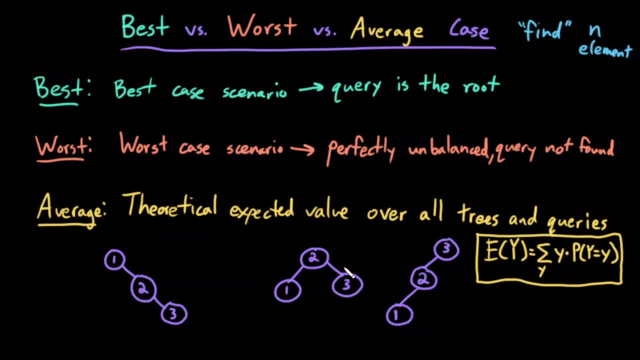 I'm looking for, I succeed Here. if I'm looking for node two, node two is the root, So immediately I succeed. And here the very first node. if I'm looking for three, I would find it immediately, So I would succeed. 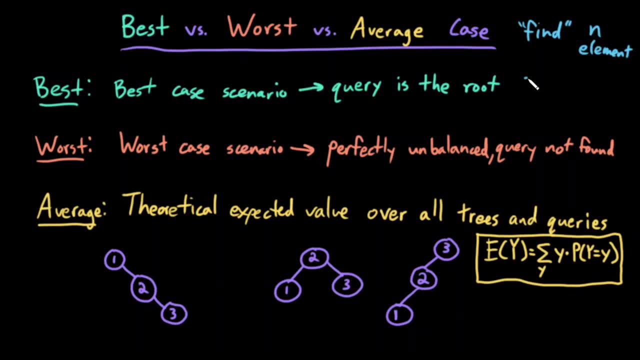 So the best case time complexity for a binary search tree is big O of one, regardless of what the shape of my tree is, And even if I have some large n elements, I will always find it when I check the root. So the best case time complexity, regardless of how large the input size is, is always 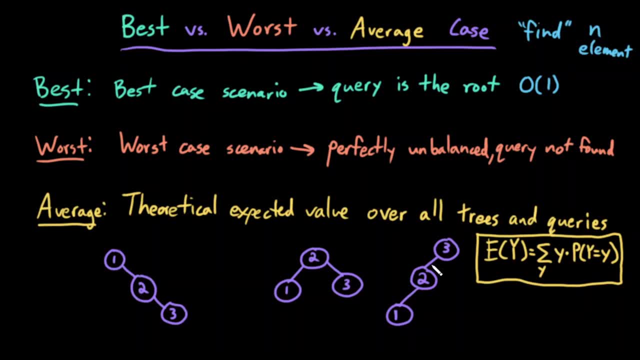 just constant time, no matter what my tree shape, is The worst case: time complexity. I have to think of the worst possible scenario which, for the case of a binary search tree, would be a perfectly unbalanced tree. So this tree and this tree, the two perfectly unbalanced trees here, are the worst possible. 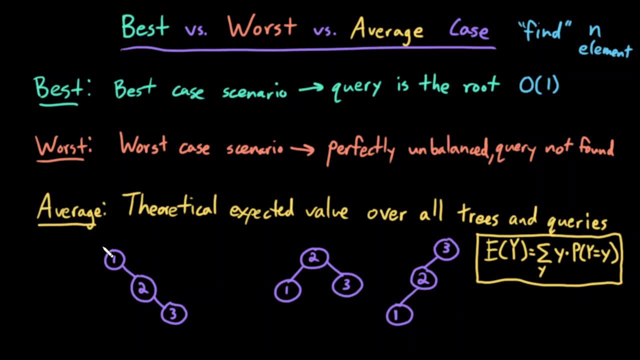 scenarios for my binary search tree find algorithm. So in this tree, if I looked for the element four, I would theoretically have to traverse over big O of n edges before I fail. And here, if I was looking for the element zero, similarly I would have to traverse. 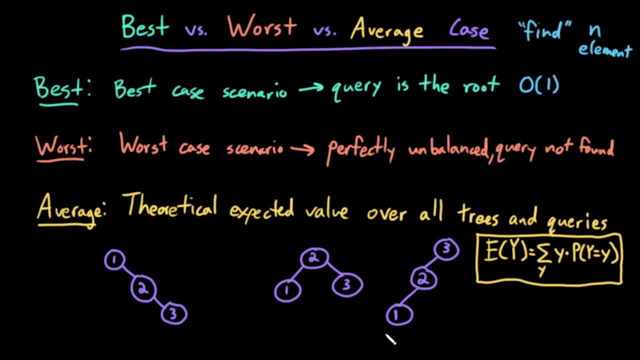 over big O of n edges before I fail. So the worst case scenario for a binary search tree is if my tree is perfectly unbalanced and I didn't find it, Or, equivalently, if it was the last element, this would be big O of n. 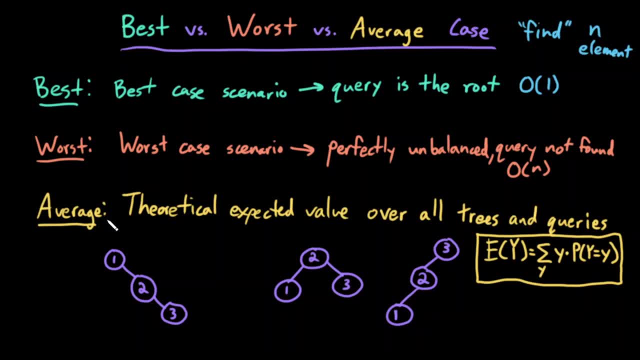 What about the average case time complexity? This is something that we don't talk about too often, but this is what we would theoretically expect. So this is the theoretical expectation. It's an actual statistical expected value over all possible scenarios we might face. 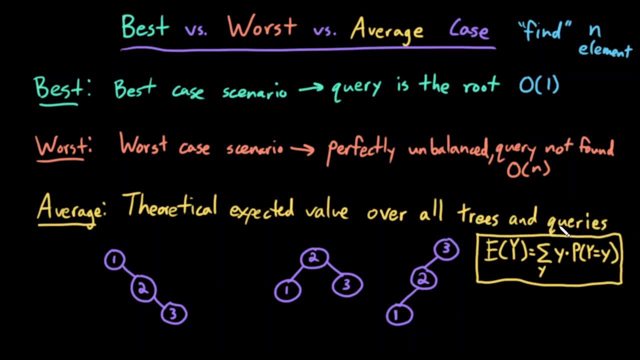 So, over all possible trees And all possible queries, it would be the expected value. And just to remind you, this is the expected value equation. So for some random variable capital Y that can have any value lowercase y, the expected value of capital Y is lowercase y times the probability that capital Y variable equals. 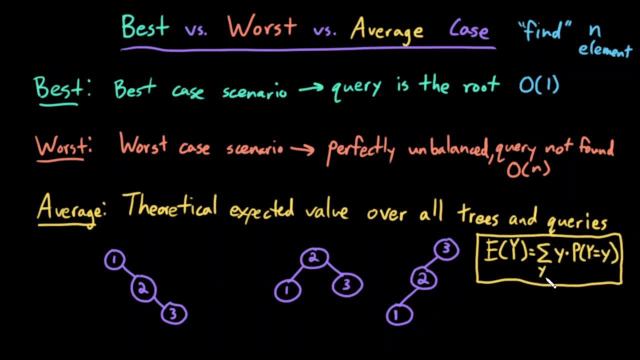 that lowercase y over all theoretically possible values. lowercase y. This seems a bit abstract, but we'll dive into it a little bit slowly. for a binary search tree, We'll talk about what assumptions we have to make and how we can actually do some form. 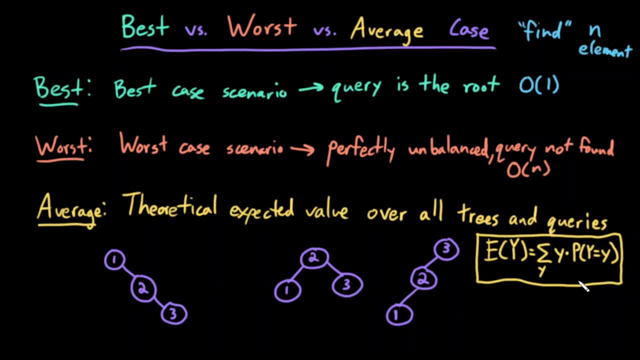 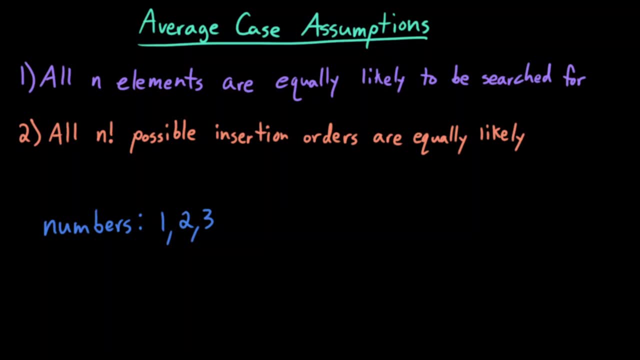 of a theoretical expected value over binary search tree shapes and queries. In order to explore the average case time complexity of finding an element in a binary search tree, I first have to make two simplifying assumptions. First, I will assume that all n elements that are in my binary search tree will have the 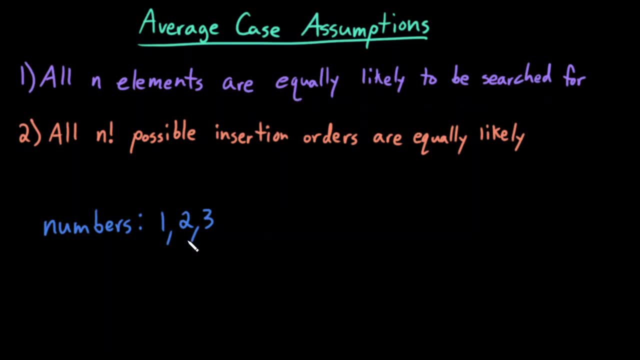 same probability that my query is 1, is the same as the probability that my query is 2, is the same as the probability that my query is 3, which, generally speaking, would mean each of their probability is 1 over n, Which, in this example, I have 3 elements. 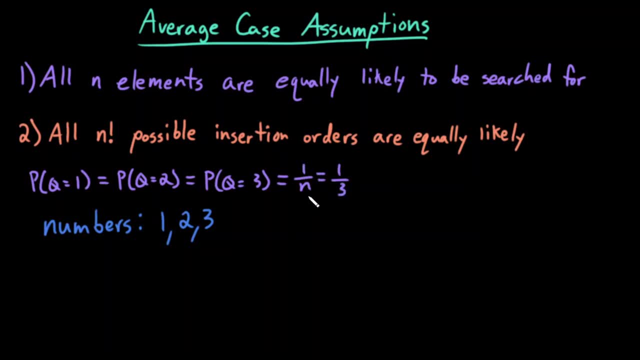 So 1 third. So I'm assuming if I have n elements, the probability that I'm searching for any specific element is 1 over n. The second simplifying assumption is that all n factorial possible insertion orders are equally likely. So, given n elements, I can pick any of those n elements to be the first one to insert. 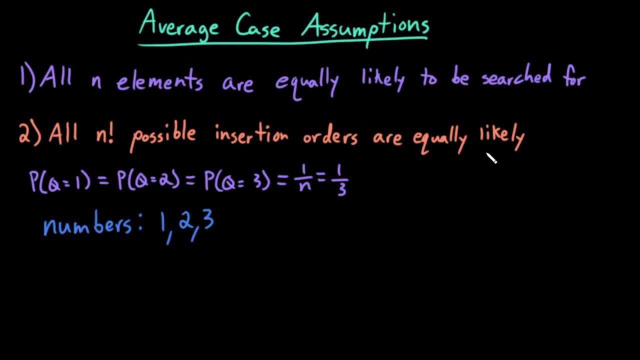 Then, out of the remaining n minus 1 elements, I can pick any of them To be the second one that I insert. out of the remaining n minus 2 elements, I could pick any of them to be the third element to insert, etc. 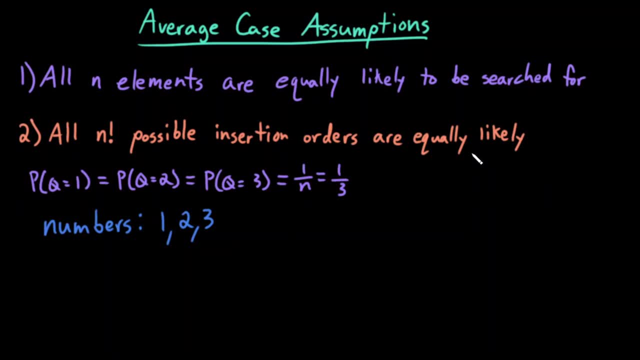 So the number of possible insertion orders, how many different orders I can actually insert n elements. there's n factorial possible ways And I'm assuming each of those is equally likely. So for this example, where I have the numbers 1,, 2, and 3, let's take a look at those. 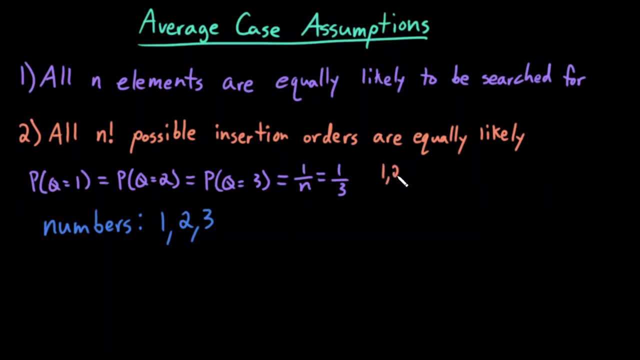 possible scenarios. So I could do 1, then 2, then 3.. Then I could do 1, then 2, then 3.. Then I could do 1, then 2, then 3.. So that would be. 1 is the root. 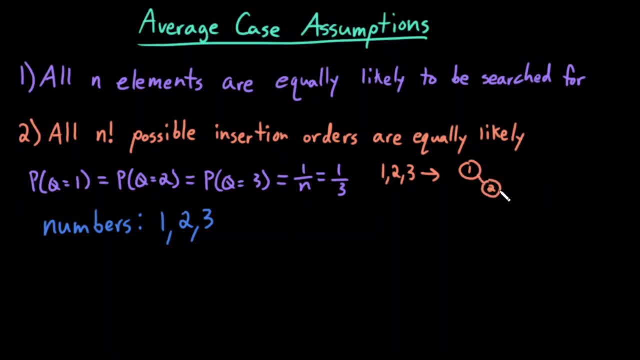 Then I insert 2.. That would be the right child of 1.. Then I would insert 3.. Oh, 3 is greater than 1.. 3 is greater than 2.. That would be the right child of 2.. 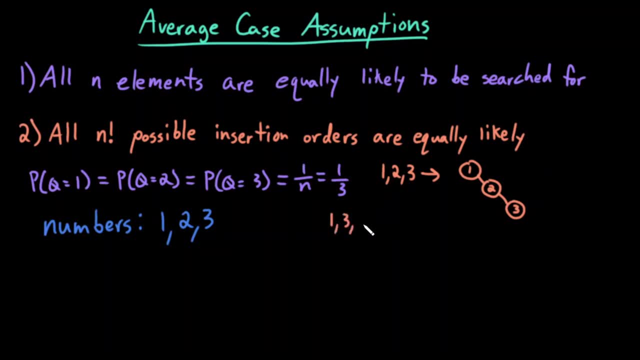 I could do 1,, 3, 2.. So 1 is the root, Then 3 is greater than 1.. So I would make it the right child of 3.. Then 2 is greater than 1.. So I traverse right. 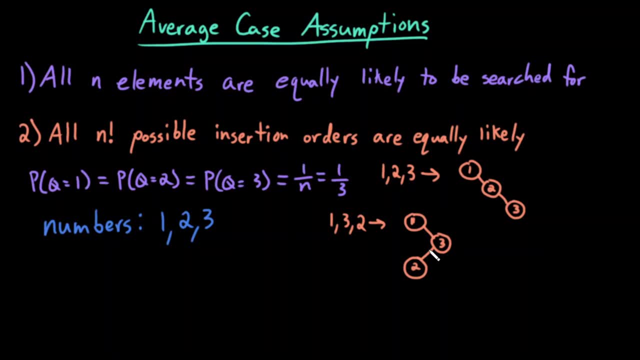 It's less than 3.. So it's the left child of 3.. I could have 2,, 1, 3.. So 2 is the root, 1 is less than 2.. So it becomes the left child. 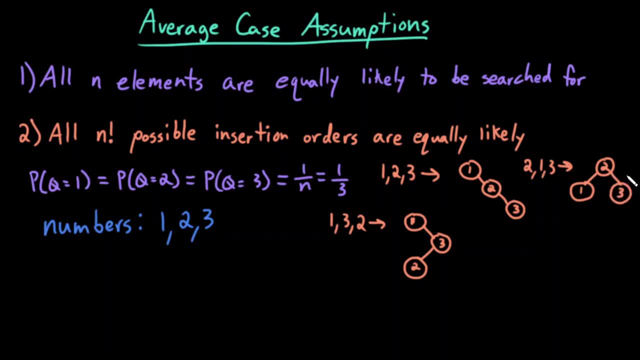 3 is greater than 2.. So it becomes the right child. I could have 2,, 3,, 1.. Which is the right child? 3 is greater than 2.. Which starts with 2 as the root? 3 is greater than 2.. 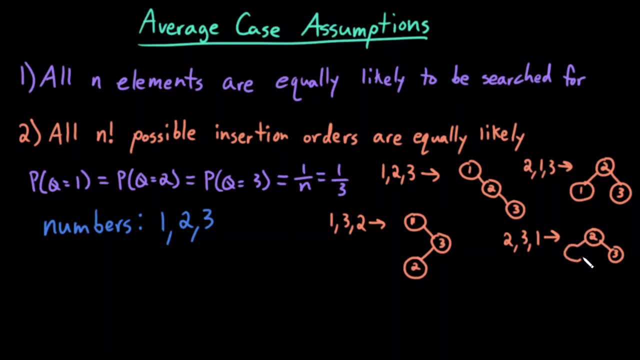 So it's the right child. 1 is less than 2.. It's the left child. I can have 3, 1, 2.. So I first insert 3., Then 1 is less than 3.. So it's the left child of 3.. 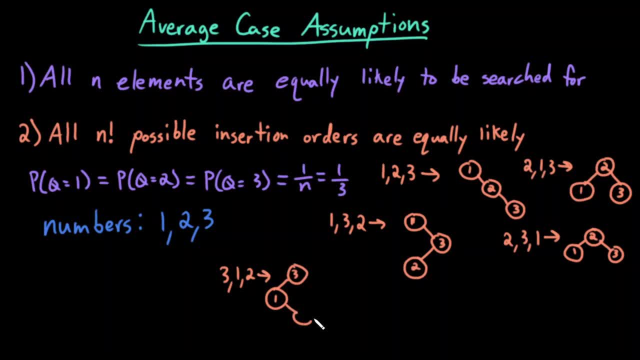 And then 2 is less than 3.. But it's greater than 1.. So it becomes the right child of 1.. Or I could have 3, 2, 1.. 3, 2, 1.. So 3 is the root. 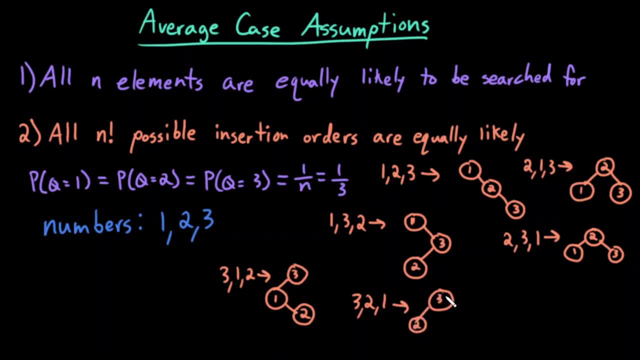 Then 2 is less than 3.. So it's the left child of 3.. Then 1 is less than 3.. And it's less than 2.. So it would be the left child of 2.. So given n equals 3, I have n factorial equals 3 factorial equals 3 times 2 times 1 equals. 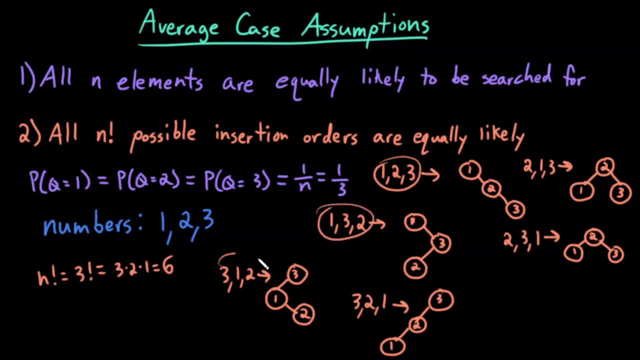 6 possible insertion orders. So I have n- factorial equals 3 factorial equals 3 times 2 times 1 equals 6 possible insertion orders, Each of them being equally likely. Notice that I'm not saying that all possible trees are equally likely. 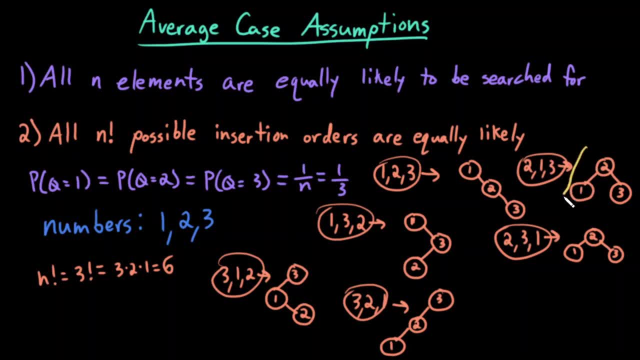 On the contrary, we see that these two different insertion orders gave me the exact same tree. When I insert 2, then 1,, then 3,, versus when I insert 2, then 3,, then 1,, I get the exact. 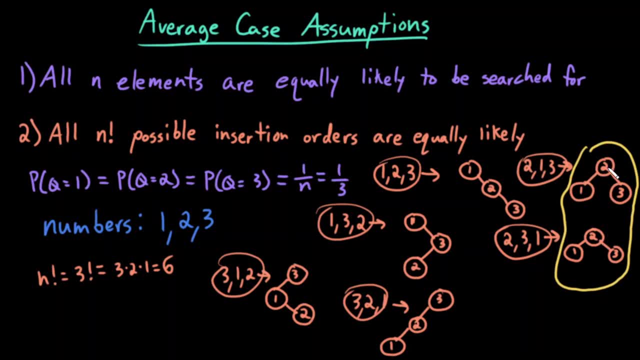 same tree. I'm not saying that all trees are equally likely. I'm saying all insertion orders are equally likely. So in this example I have 1,, 2,, 3,, 4, 5 unique tree shapes, but this tree shape is twice. 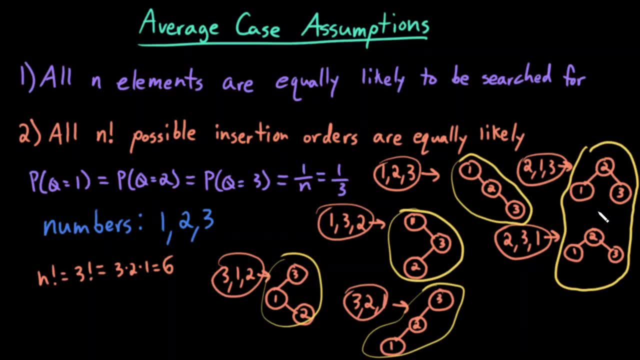 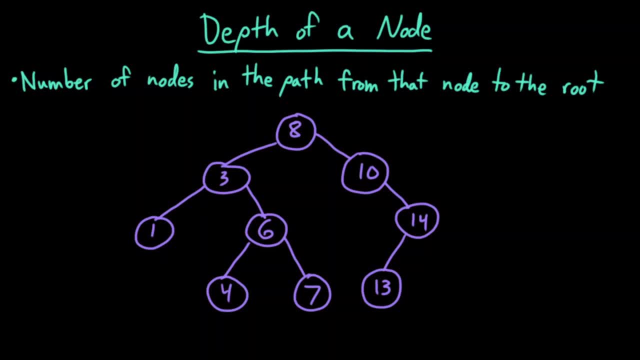 as likely as the other ones because there was two different insertion orders that gave rise to it. Let's also introduce the concept of the depth of a node. We will define the depth of any given node to be the number of nodes in the path from. 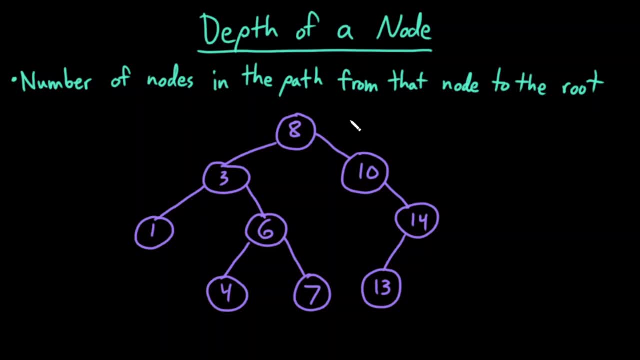 that node to the root. So for example, in this tree let's label all the depths of each node. So for the root, the number of nodes from the path from the root to the root is just one node itself. right, It is the root. so the number of nodes between 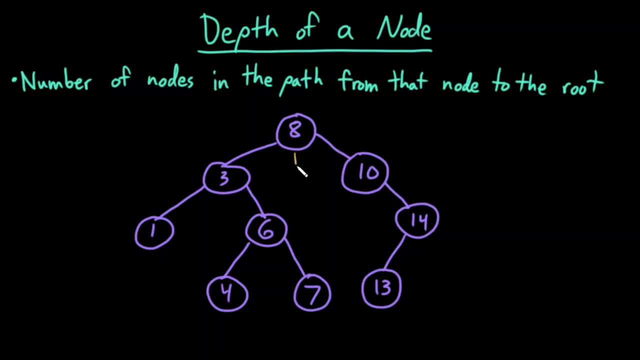 it and the root is itself. So just one here. What is the depth of this node? Well, there's one, two nodes on the path from this to the root, so its depth is two. For 14, there's one, two, three nodes along the path to the root. For node 13, there's one. 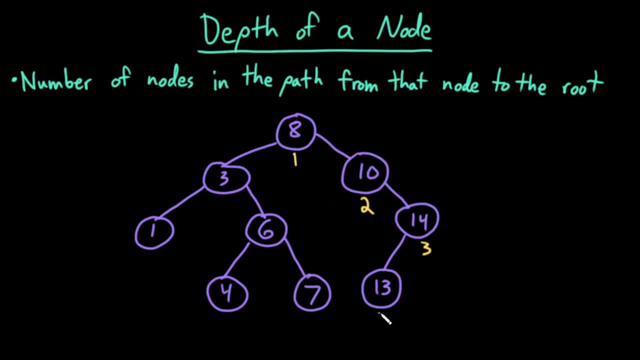 two, three, four, five, six nodes along the path from it to the root. Here there's one, two nodes, One, two, three, One two, three. One two, three, four. One two, three, four, And now we've labeled the depth. 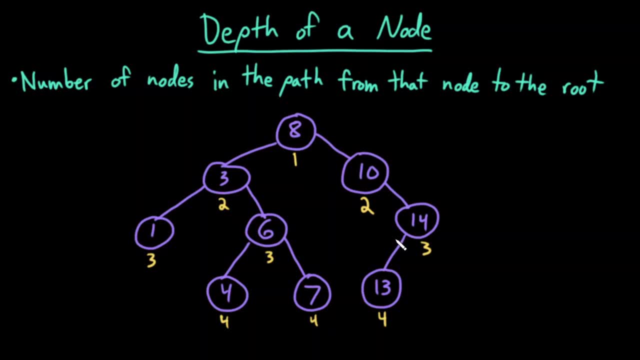 of every single node. So why did I just introduce this new term? Well, if we think about it, we're trying to compute the average case time complexity. So average case time complexity, It's the expected number of operations to find a query. 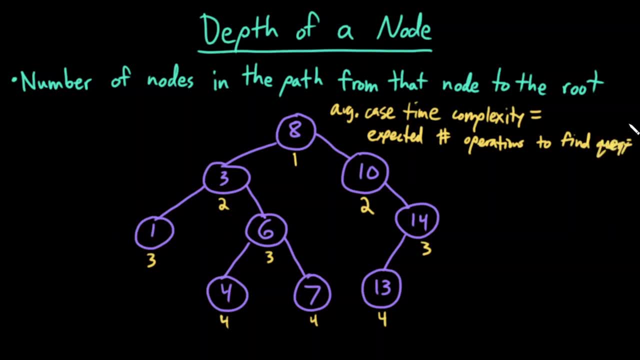 qu? ery. So the expected number of operations to find a query. So let's say one operation is one comparison. Let's say I was looking for the number three. I would compare three with eight. Oh, three is less than eight. Let me go left. I would compare three with three. Oh, they're equal. 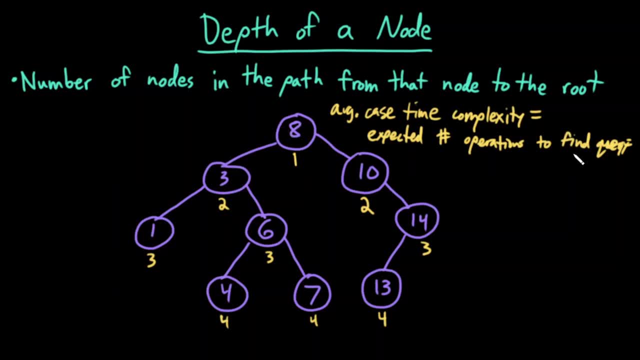 I've succeeded. So that would be two comparisons And the average case time. complexity is the expected number of operations to find a query. So let's say I was looking for the number three. Oh, three is less than eight. Now let's say I'm gonna look around. I have a question. 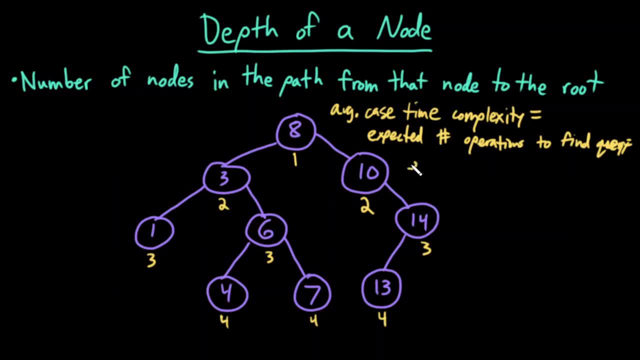 here. So I went to this and I said: Of course we're gonna compare 3, 8,, 9 to 8.. When you compare 8 to 8, you do the same thing. What do you still did? So I went from 3 to 8.. So 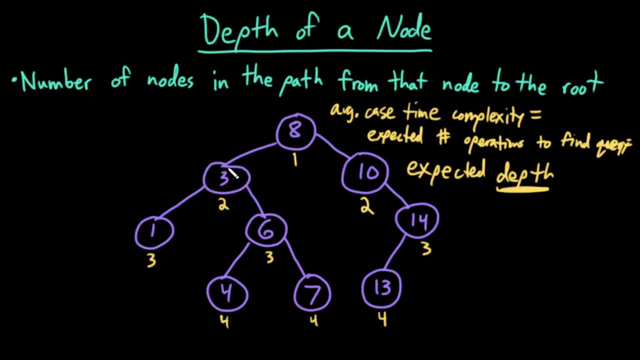 define 3 to 8.. So three is equal to 3, and then I went up to twoorders. Let's say I was looking foraciones to find. Let's say I was looking for the number 13.. 13 is greater than eight. that's one comparison. 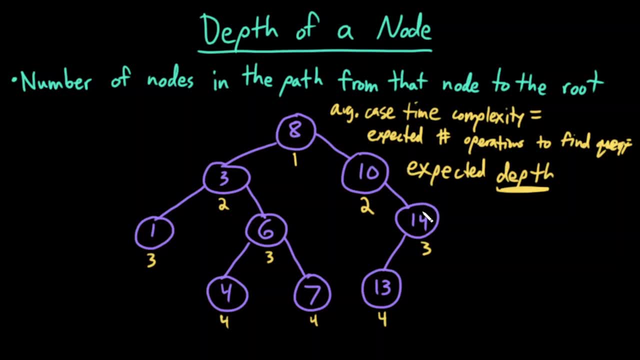 13 is greater than 10, that's a second comparison. 13 is less than 14, that's three comparisons. 13 equals 13,, that's four comparisons, which is equal to its depth. So, generally speaking, the number of comparisons. 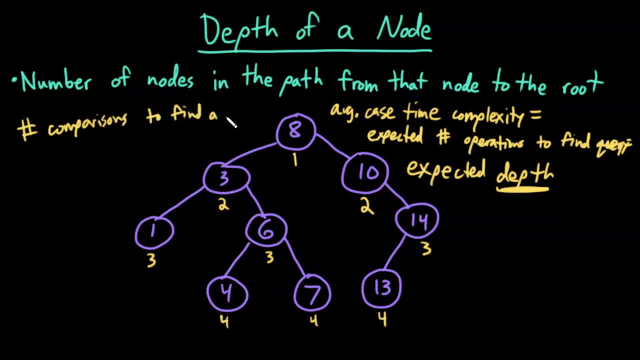 to find a node is equal to the depth of that node, which is why we're able to make this jump. So average case time complexity being the expected number of operations to find a query. that's just the definition. So this here is the definition. 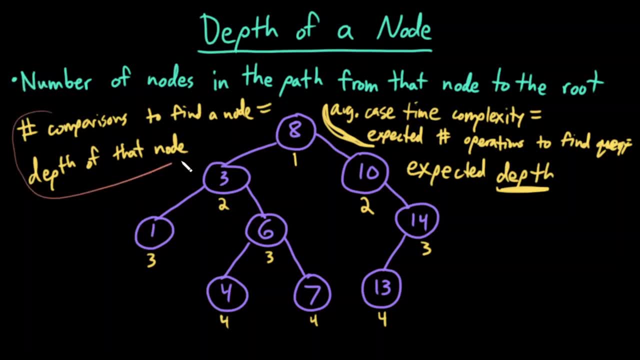 But then, given this piece of information, this realization that the number of comparisons to find a node is just the depth of the node, we can now translate average case time complexity into this. It's just equivalent to finding the expected depth over all possible nodes. 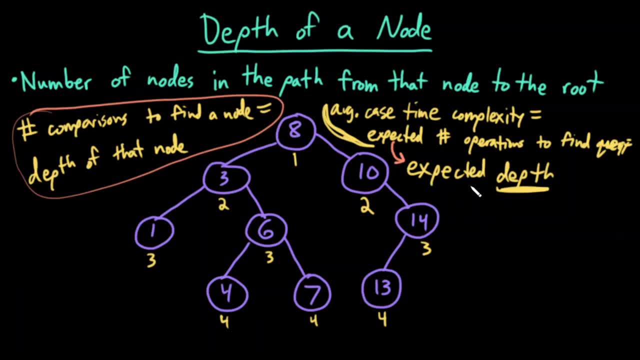 What is the expected depth? Well, expected depth, it's an expected value of the depth. So let's say that the depth of some given node, X, is D, of X the expected value of depth. so expected value of, let's say, D. 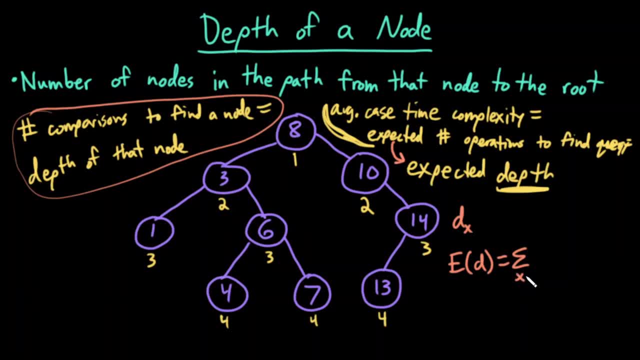 is the sum over all possible nodes X of the depth of X times the probability that I'm looking at this. so my query is X And remember previously I told us that all possible queries are equivalent in terms of probability. So this is the same thing as the sum over all possible queries. 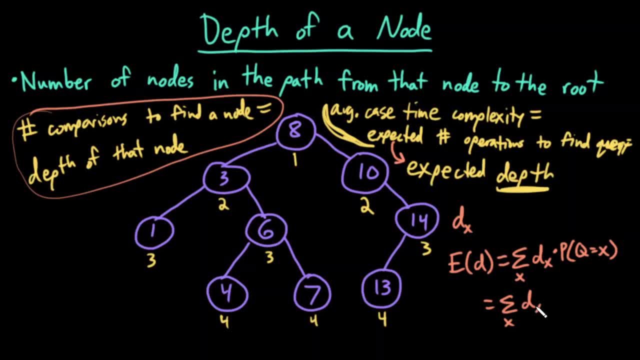 or all possible nodes X of the depth of that node times one over N. right, I have N possible nodes. They're each equally likely to be searched for, So the probability of any given node X is one over N. I could pull this out of my sum. 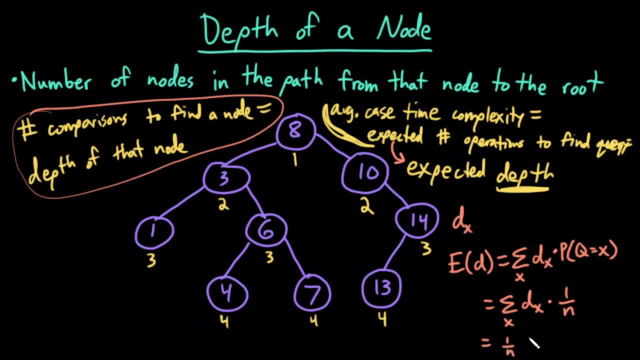 This equals one over N times the sum over all possible nodes X of the depth of X. This is not DX like in calculus, This is D subscript X. so the depth of X. So, in other words, if I can find the sum over all nodes X, 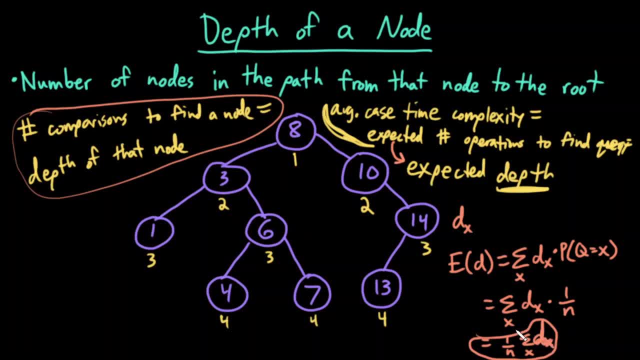 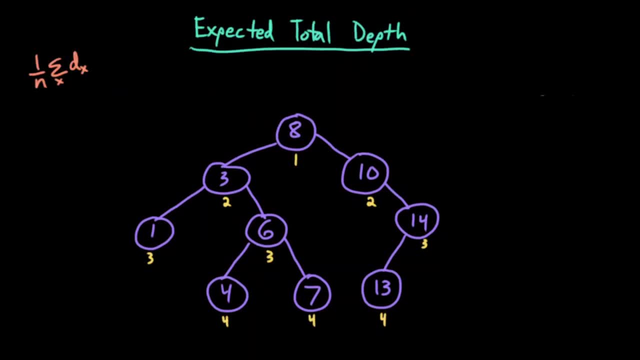 of the depth of that given node. I would just multiply that by one over N and that would give me my expected value. So we figured out that the average case time complexity of finding an element in a binary search tree is just the expected depth of a node. 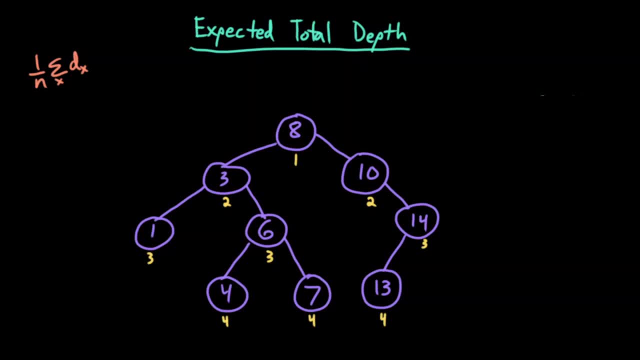 in a binary search tree which, assuming all nodes are equal, all nodes are equally likely to be searched for, is just one over N times the sum of the depth of all of the nodes in that tree. But there's one big issue here. This equation is- assuming that I'm only looking. 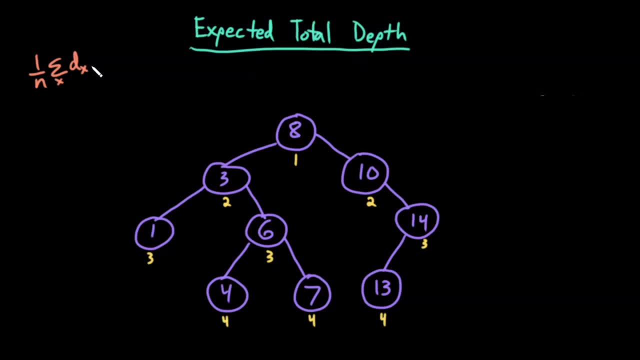 at a specific single binary search tree. However, the expected value that I'm looking for, the average case time complexity- should be over all possible scenarios, which means all possible insertion orders. So to tackle that generalization, let's talk about what expected total depth would be. 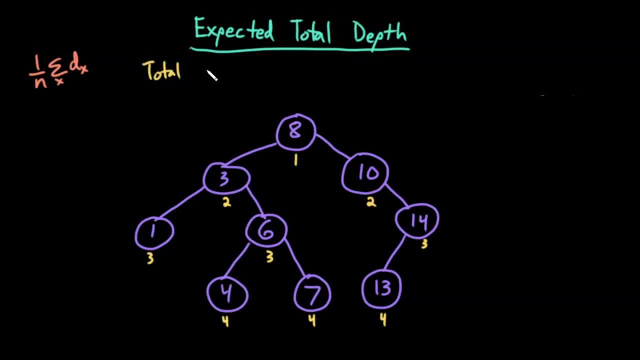 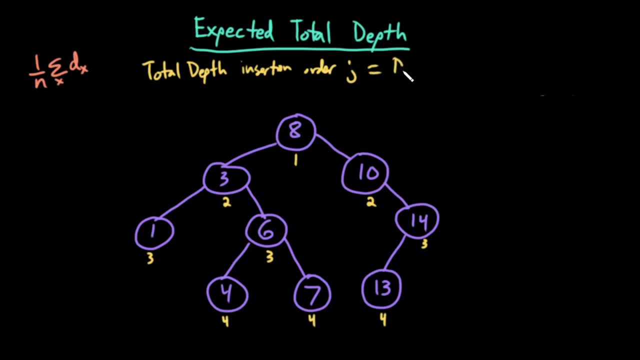 what does that predetermine? It'll remind me of some of this last drain that I learned from class talking of N, but I'll keep in mind N in the transitions. So this actually examples the final depth of an insertion order J. in order to know exactly the final depth. 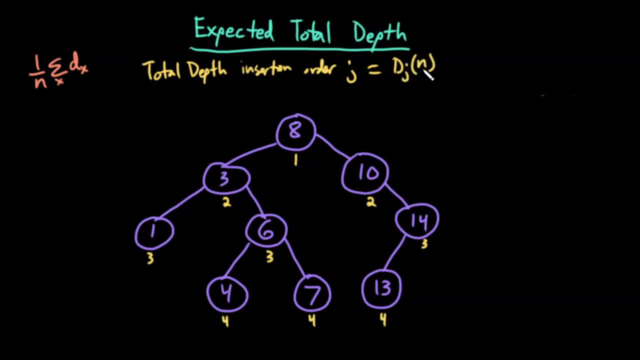 which we call n factorial. So for that past prompt system we can sort of make the meaning of: that is higher than N Theyनse. each of them is higher for this terms. So we apply that function and finally this: JEN孤Nї� deliverdle. 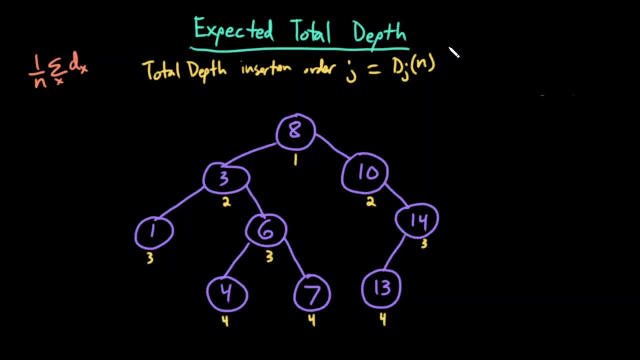 called N, factorial possible insertion orders is total depth across all possible insertion orders. Therefore, let's let- I'll use a different color for this- let's let d of n, so no subscript j- be the expected value over all possible total depths for specific insertion orders. So this would be the sum over all possible. 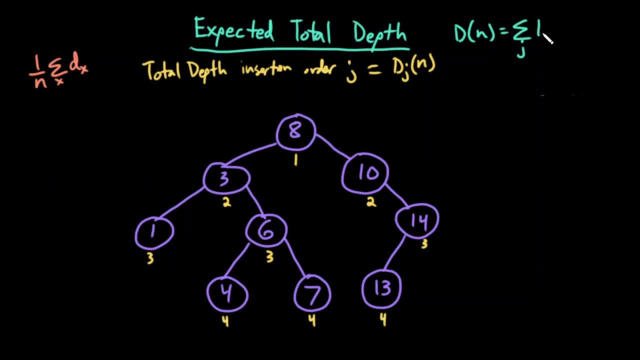 insertion orders j of the total depth, given that insertion order times the probability that I actually saw that specific insertion order. so the it it's the total depth of insertion order j times the probability that I inserted my elements in insertion order j. but remember my set full insertion order is s all certain, so it was one old set for j over, so j is I. 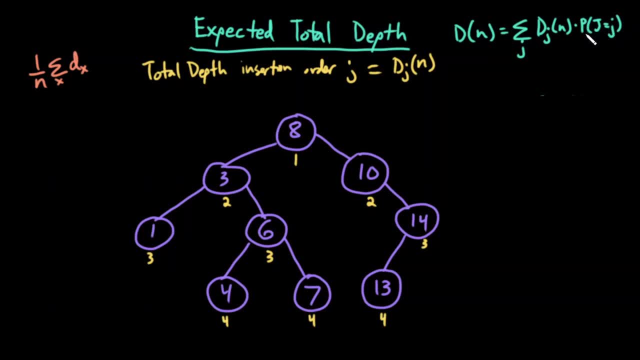 second assumption was that all insertion orders are equally likely. Therefore this probability here, the probability that I specifically saw, insertion order little j is just 1 over n factorial. There's n factorial possible insertion orders. They're all equally likely. So the 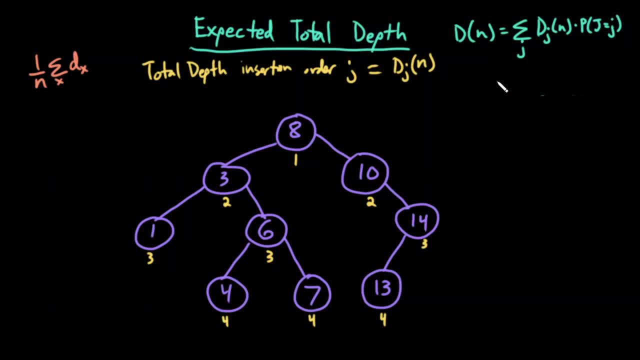 probability of this specific one is 1 over n factorial. So this becomes the sum over all possible insertion orders j of the total depth of insertion order j times 1 over n factorial. I can pull this out of my sum, So the expected total depth would be 1 over n factorial times. 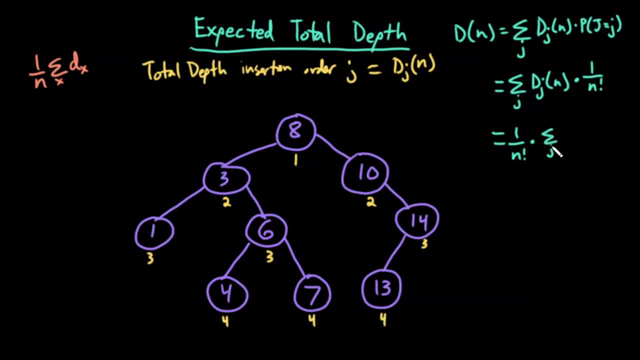 the sum over all insertion orders j of the total depth of insertion order j. So I'll say j equals 1 to n factorial because there's n factorial possible insertion orders j. So hopefully that follows. Let's just recap real quickly. So we said total depth of a given tree. 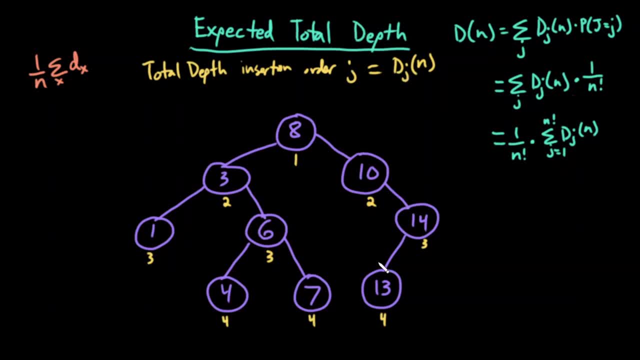 is. So the total depth of a specific tree is just the sum of the depths of all the nodes. So just real quick, to make sure people are following what that means: The total depth of this tree is the sum of the depths of all the nodes. So the total depth of this tree is the sum of the nodes. 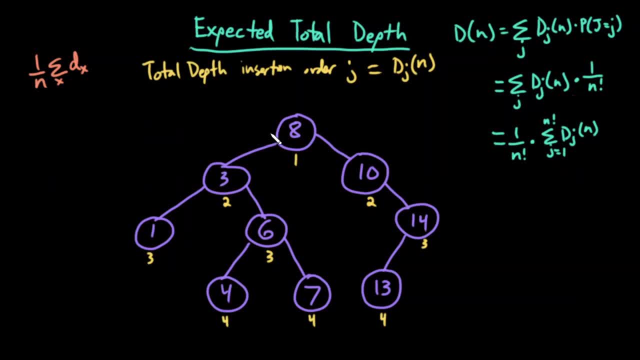 Let's say, this tree was created using insertion order. Well, let's not worry about that. So for this specific tree, the total depth is 1 plus 2 plus 2 plus 3 plus 3 plus 3 plus 4 plus 4 plus 4, right, I'm just adding the depths. 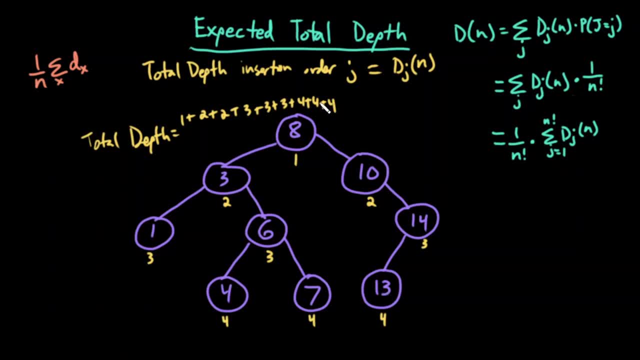 of every single one of these nodes. So this is 4,, 8,, 12,, 15,, 18,, 21,, 23,, 25, 26.. So, if I'm doing my math right, which hopefully I am, the total depth. 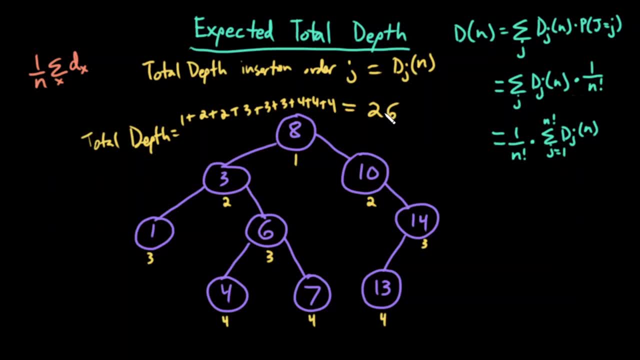 of this specific tree is 26.. So the total depth of an insertion order j is the sum of the depths of all the nodes of the tree resulting from that insertion order, And the expected total depth is 1 over n factorial times the sum of the total depths of every single possible insertion order. 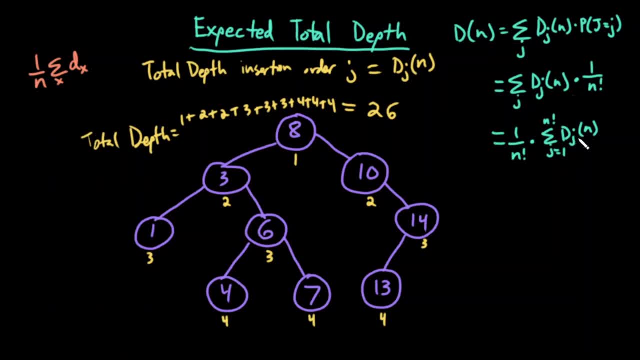 Okay, so this sounds like I've just done something bad. I basically have determined our answer with respect to some n factorial sum. Do I actually have to enumerate all possible n factorial insertion orders and compute the total depth of every single one, Or can I do something to rethink? 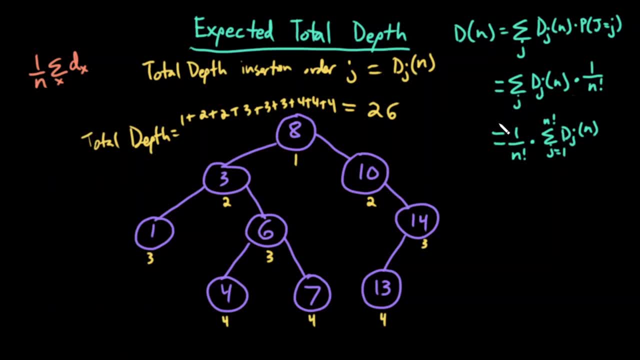 this and maybe make my computation work. So I'm going to do this, I'm going to do this, I'm going to do this. Let me figure out what this element is that I want, And I think I know how to do it. 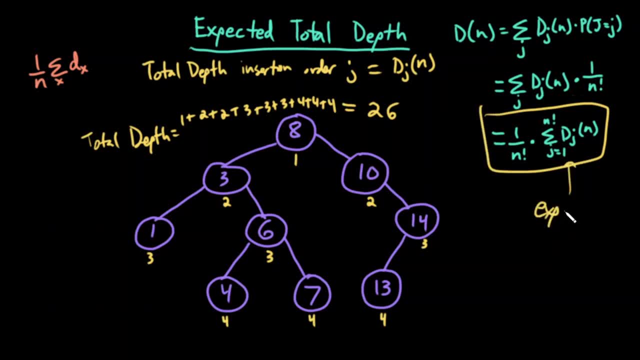 but I need to figure out what r is equal to n and k it. So I'm going to pull this here, So I am going to loyal the linear representation and voting at the object, at argument level, on my bölth. So that way if I'mкийing, if I'm plotting a n variable on both sides together, 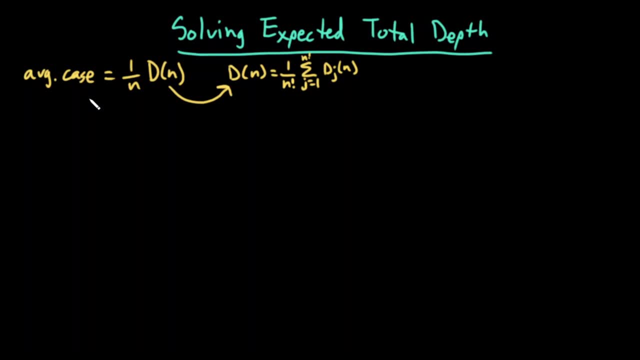 I normally have and unitary type sz object. What I'm doing is I want to go with the information that I want to tell you about the n variable and I need an taking away variable. So, for example, likely to be searched for. I made this equal to 1 over n, so 1 over the probability of searching. 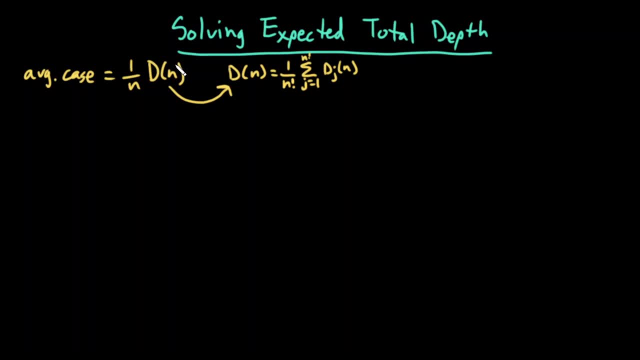 for any given node times the total depth of a tree with n nodes. So the expected total depth of a binary search tree with n nodes? If I could find this out I would have my answer. So the expected total depth of a binary search tree with n nodes? well, using assumption 2,. 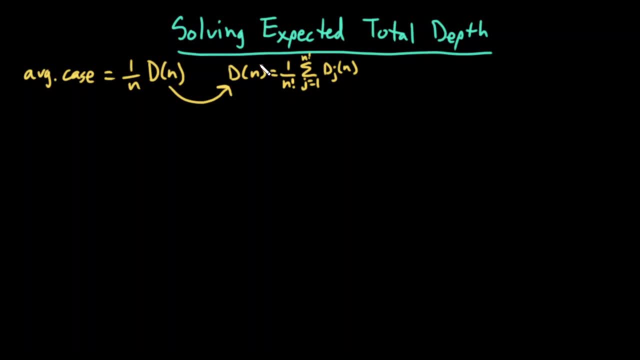 I figured out that I'm assuming all insertion orders are equally likely. Therefore, over all possible n factorial insertion orders, the expected total depth would be 1 over n factorial. the probability of seeing a specific insertion order times the sum of the total depth of 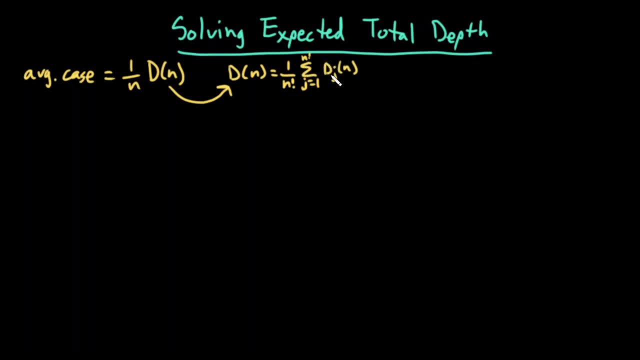 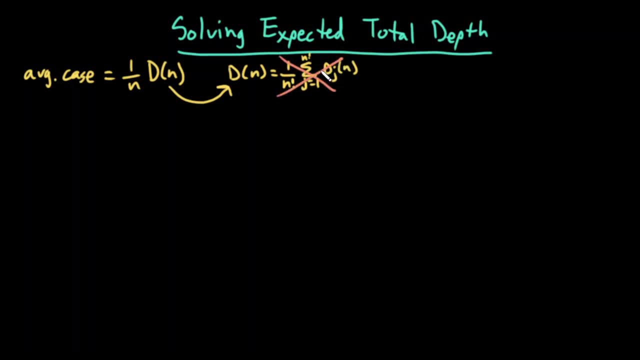 sum, So hopefully I can avoid doing this. Is there some better way of computing the expected total depth of a binary search tree with n nodes without having to do this exponential sum? Let's try to think of a general scenario. So let's imagine a binary search tree. 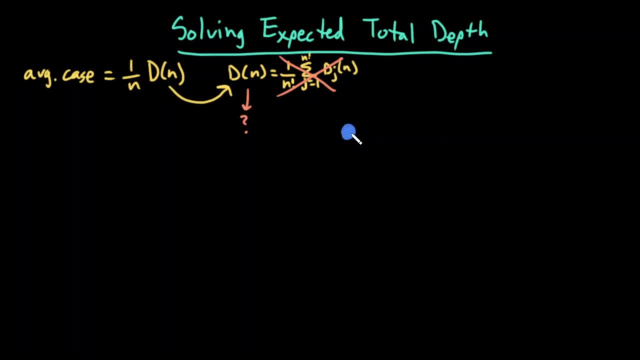 that has n nodes in it. It has a root And let's say it has i nodes in its left subtree. If it has i nodes in its left subtree, it must, by definition, have n minus i minus 1 nodes in its right subtree Because, remember, there's n elements total. 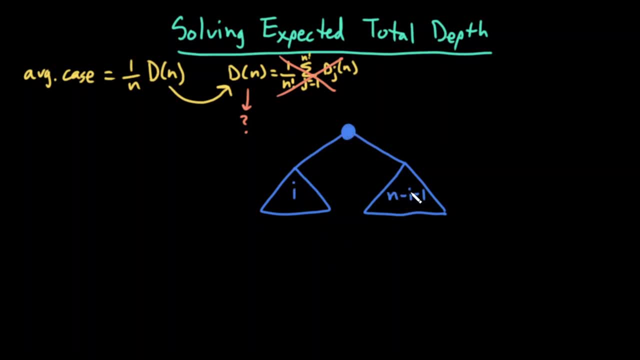 so 1 plus i plus, n minus i minus 1 is n total. So let's define d of n given i is the expected total depth of a BST with n nodes total and i nodes in its left subtree. So, in other words, let's let d of n given i be the expected total depth of this tree. 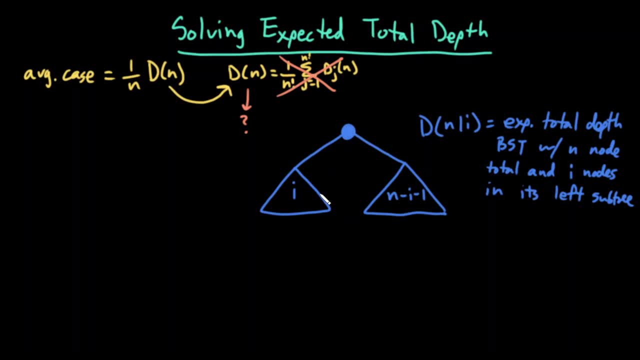 here. It has a root and it has i nodes in its left subtree and there's n nodes total. Let's think of this recursively. How can I define this recursively? I can actually define d of n given i as a function of d of n given i. 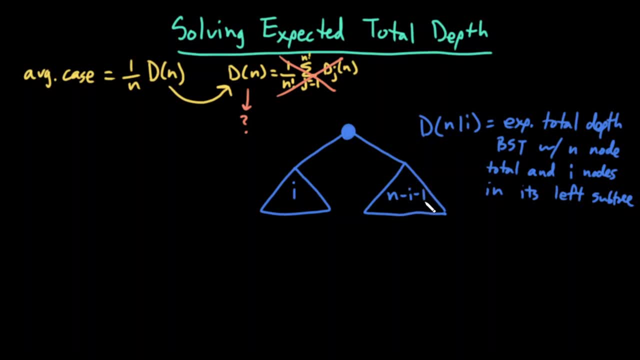 of d of i and d of n minus i minus 1.. So this itself was a tree. This itself is a valid binary search tree. Just this subtree here. It's a valid binary search tree. It has some depth, i. So d of i. 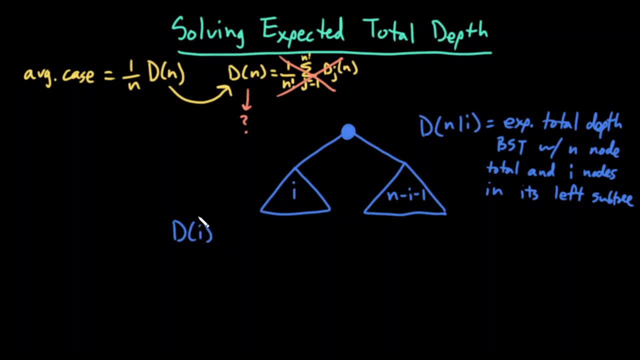 is the expected total depth of a binary search tree with i total nodes. This is the expected total depth of a binary search tree that has n minus i minus 1 nodes. These are just the definitions of what d of i and d of n minus i minus 1 would be If I had. 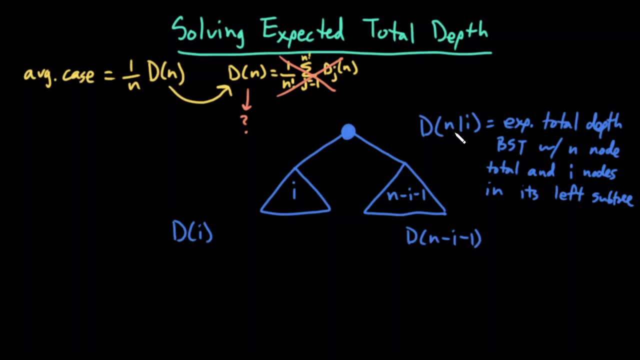 these two values, I could find d of n given i, because it would be So. d of n given i would just be The expected total depth of this subtree plus the expected total depth of this subtree, plus I've added one to every single node in here's depth, So each node here is now one node further. 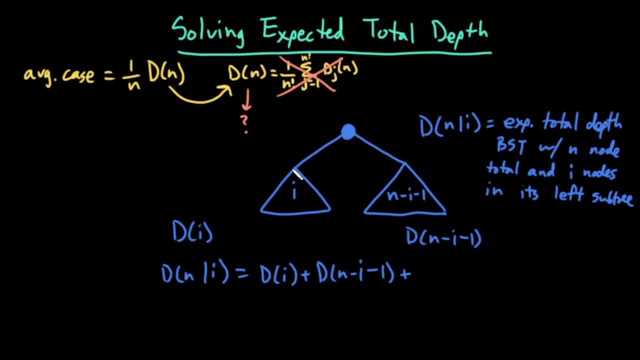 from the root, because I've added this new root, So let's say the root of this subtree. it used to have a depth of zero, but now that it's become the subtree of this overall tree, its depth has now increased to one. Its child's depth has increased to two. So every node. 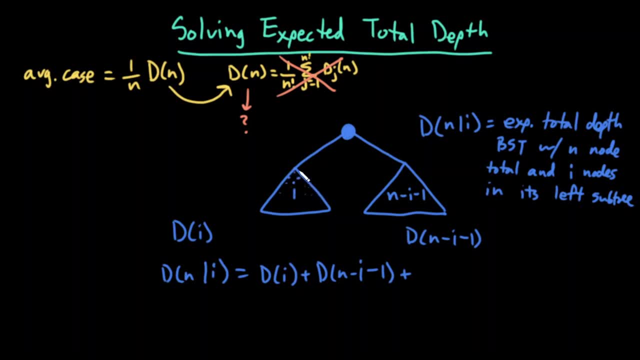 in this subtree. by attaching this subtree as a child of this root, its depth has increased. So I add one for each of my i nodes here. So I add i in total. And similarly, each of the n minus i minus one nodes in this subtree now has one larger depth. So for each of these nodes, 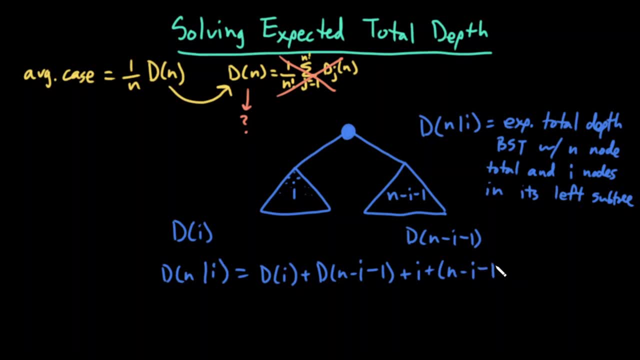 each of these n minus i minus one nodes, I've increased my total depth by one. So I increase my total depth by n minus i minus one in total, plus my root has a depth of one. Therefore the expected total depth of a. 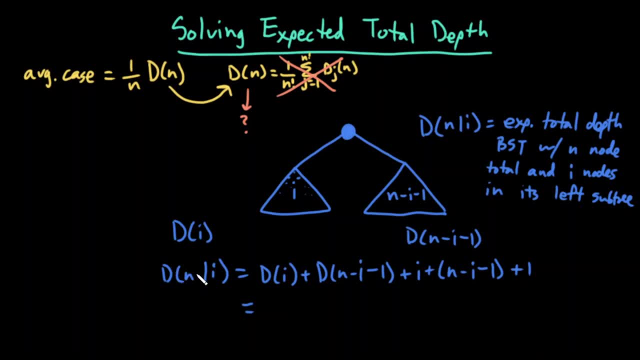 given tree. the expected total depth of a tree with n nodes, given that it has i nodes in its left subtree, is just the expected total depth of a tree with i nodes, plus the expected total depth of a tree with n minus i minus one nodes plus. so this cancels out with this. 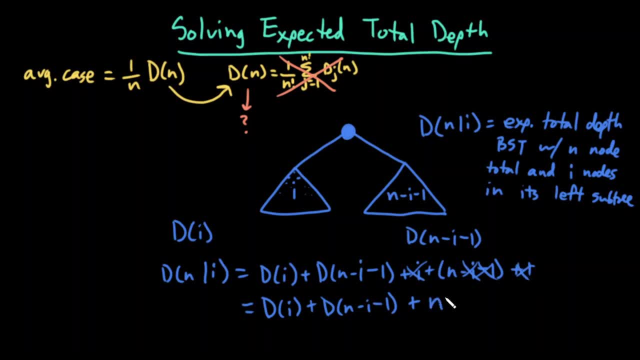 this cancels out with this plus n. So how can I use this to solve my answer? Well, basically, what is the? so the expected? so then, so d of n, which is what I'm looking for, it's this term: d of n equals the expected. 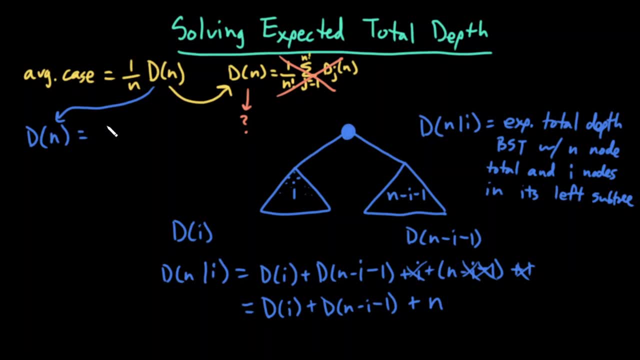 value over all possible i's. So this is: the sum over i equals zero to n minus one. I have a root. Therefore, the smallest number of nodes I can have in my left subtree is zero. That would be if all my nodes are in my right subtree. 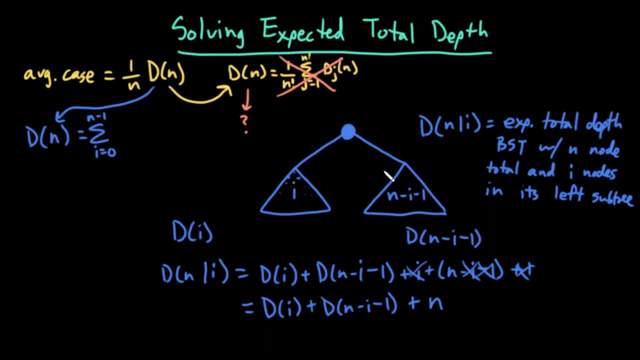 Or the largest value is n minus one. That means that I have no nodes here. So all nodes other than the root are in my left subtree. So the sum from i equals zero to n minus one of d of n, given i times the probability. 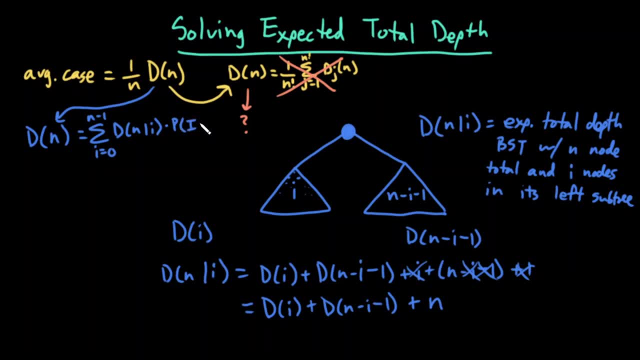 that I have i nodes in my left subtree. So it's the expected total depth of a tree with n nodes and i nodes in its left subtree times the probability of having i nodes in your left subtree. So again, I've introduced an unknown term. 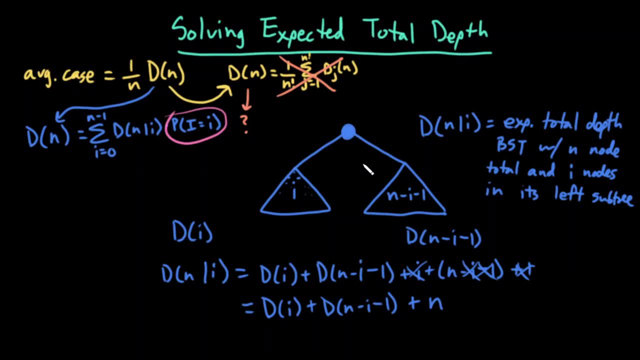 What is this? If I had this term- probability of having i nodes in my left subtree- I would be able to solve this, which means that I would be able to solve this, which means that I would be able to solve this. So what is this term? 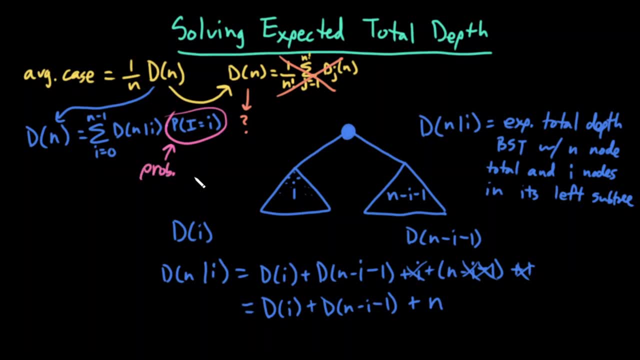 Probability. so let's reiterate: So this is the probability of having i nodes in my left subtree. This may seem confusing at first, but think about what dictates having i nodes in your left subtree. That means that the root is the i plus one. 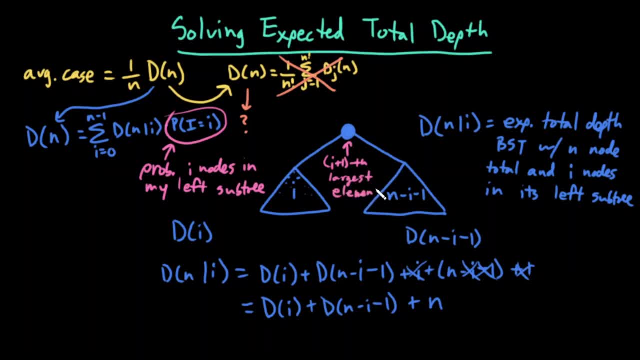 largest element. If I have n elements total, if I have i nodes in my left subtree, that means that the root is the largest element. the root is the i plus one largest element. so for example, let's say i have three, two, one and four in this example, 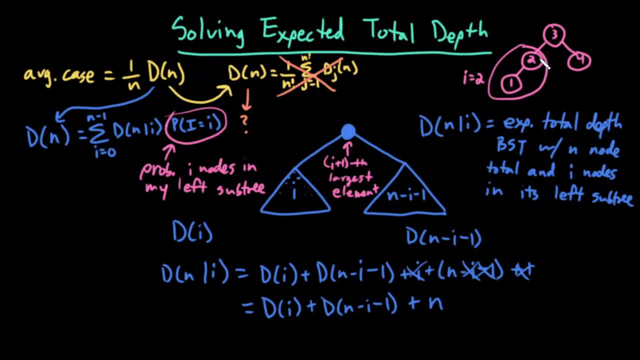 i equals two. i have two nodes in my left subtree. this came about because the root was the i plus one, the two plus one or the third largest node in my tree. so it's just some specific node in my tree and what made three be the root of my binary search? 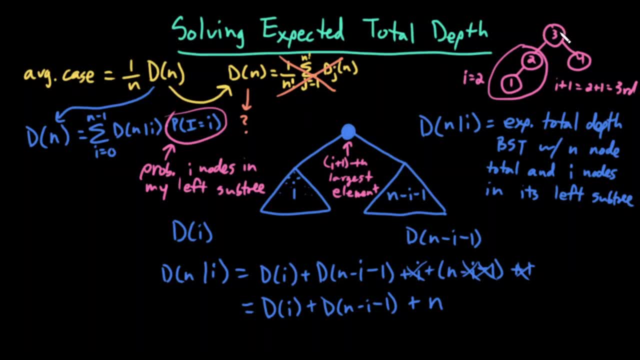 tree. well, by definition, the root of a binary search tree is the first node that was inserted. therefore, this probability, the probability that i have i nodes in my left subtree means a different color. this is equivalent to the probability that the i plus one largest or, uh sorry, smallest. 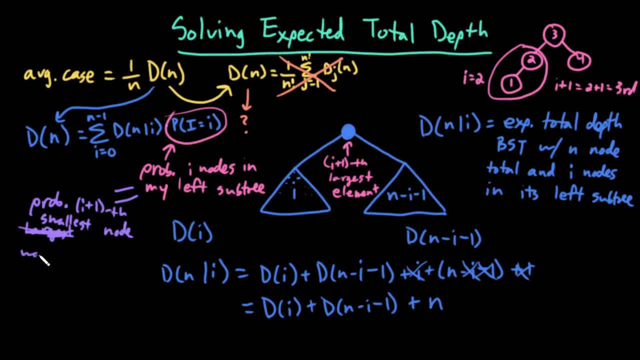 smallest node was the first to be inserted here. the probability of having two nodes in my left subtree is the probability that the third smallest- sorry, this should also be smallest. so the probability of having two nodes in my left subtree is the probability that the third smallest element was the first one that was inserted. but remember, assumption 2 said all insertion orders. 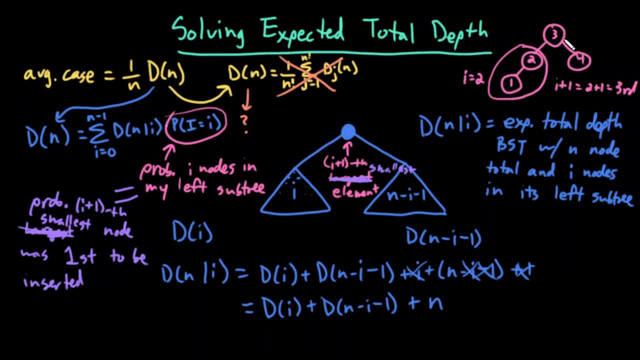 are equally likely. so out of my n possible nodes that i could have inserted first, i happen to pick this one. well, the probability of that is just one over n. the probability of first inserting any of my nodes is just 1 over n, because all insertion orders are equally likely. 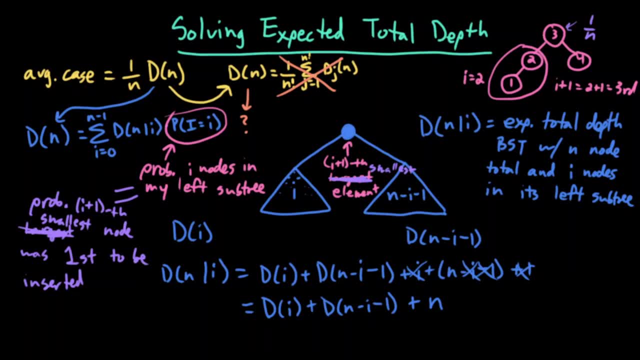 so, to finish this off, i can rewrite this as d of n equals. this probability is just 1 over n. I can pull it out: this is 1 over n times the sum from i equals 0 to n, minus 1 of this term: d of i plus d of n, minus i, minus 1 plus n. 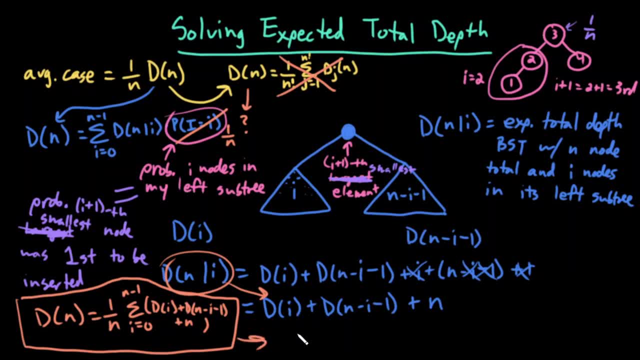 So now? so let me actually rewrite that. so that's all in one line. So just So: d of n equals 1 over n times the sum from i equals 0 to n minus 1 of quantity d of i plus d of n minus i, minus 1 plus n. 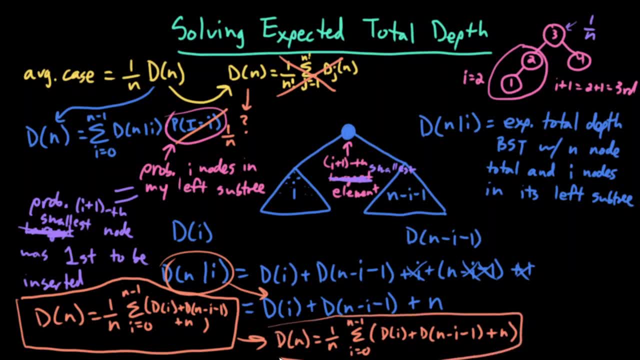 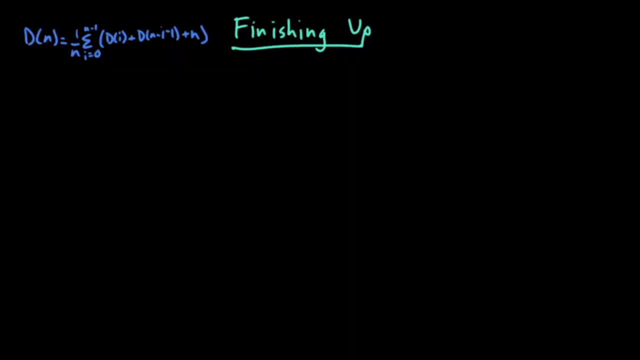 So I'll circle this one. actually it's all in one line and even though this equation, this recurrence relation, looks complicated, it's at least a closed form recurrence relation only depending on d of some input. It only depends on the expected total depth. This was quite a journey, but let's finish this up. So we last ended with a final recurrence. 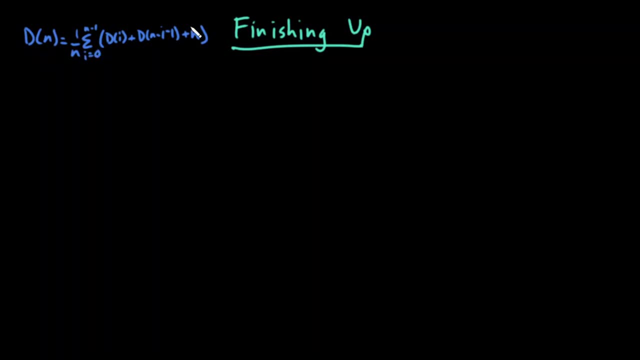 relationship for d of n as a function of all these terms over here. 1 over n times the sum from i equals 0 to n minus 1 of quantity d of i plus d of n minus 1 of quantity d of n minus 1 of. 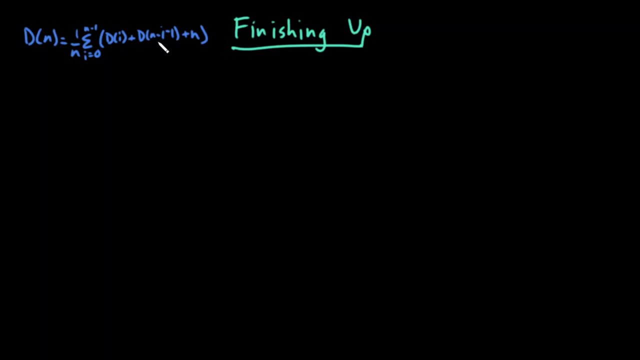 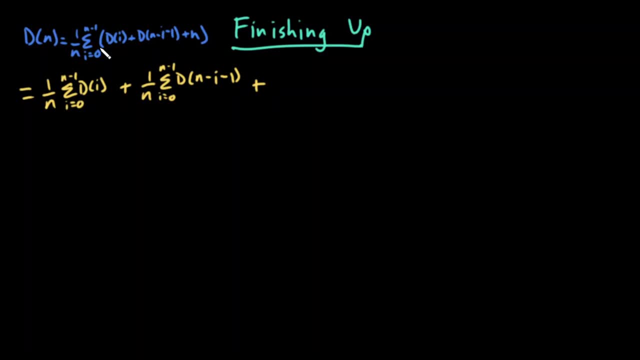 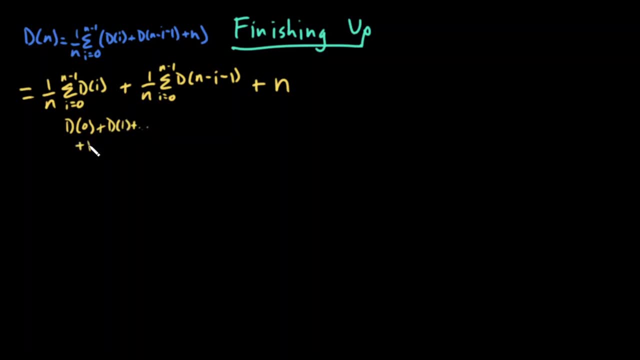 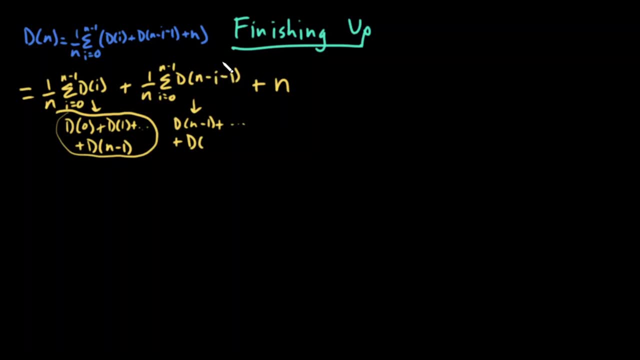 minus n minus 2 plus minus 1. so basically, when i equals n minus 2, this is just d of 1, and when i equals n minus 1, this is just d of 0. so this sum and this sum are actually the exact same sum, just solved in two different orders. 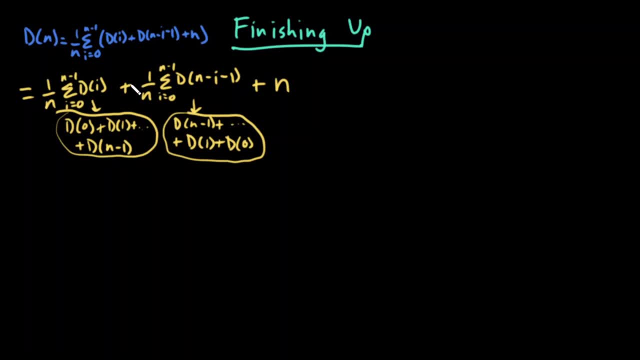 this is going from 0 to n minus 1. this is n minus 1 to 0. it's the same exact sum. so we could say that this equals basically 2 over n times this sum, because they're the same thing. so just 2 over n, just multiply by 2 and then plus n. i can multiply both sides by n, so i would get. 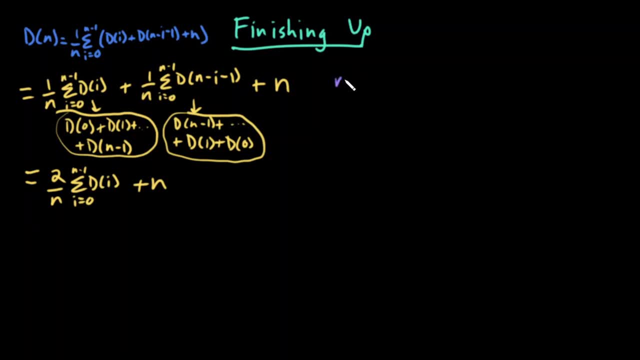 let me use a different color now. so i would get n times d of n equals 2 times the sum from i equals 0 to n minus 1 of d of i plus n squared. then i could substitute n minus 1 for n. i would get n minus 1 times d of n. 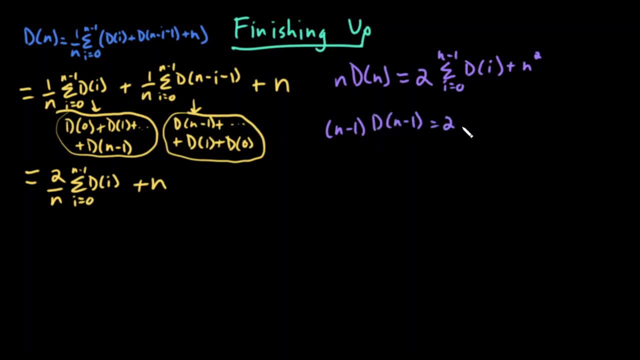 d of n minus i equals 2 times the sum from i equals 0 to n minus 2 of d of i plus n minus 1 squared, And then I can subtract this equation from the one before it and I would get n d of. 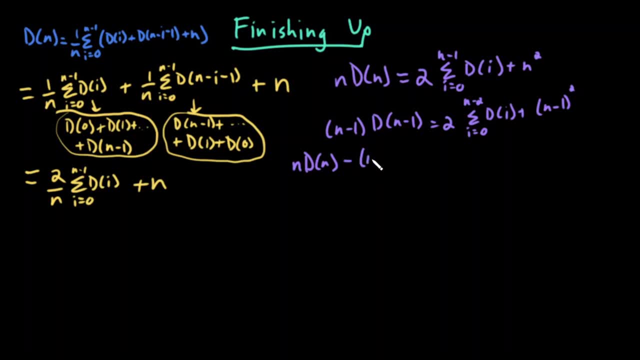 n minus n minus 1. d of n minus 1 equals 2 times d of n minus 1 plus n squared minus n minus 1 squared. If I collect these terms, I can get a final recurrence relation of- let me actually use a different color for this- of n times. 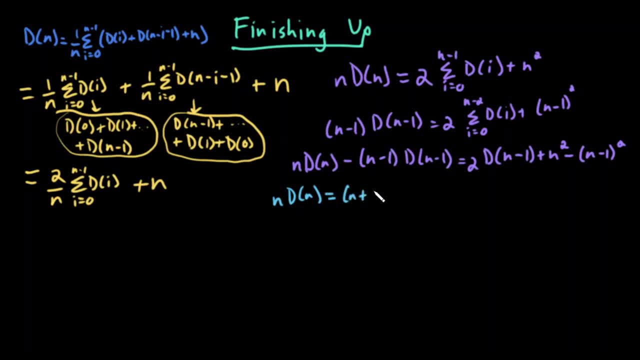 d of n equals n plus 1 times d of n minus 1 plus 2n minus 1.. And to solve this recurrence relation I can divide by n times n plus 1 to get d of n plus 1 over n plus 1 equals d of n minus 1 over n plus 2n minus 1 over n times n plus 1.. 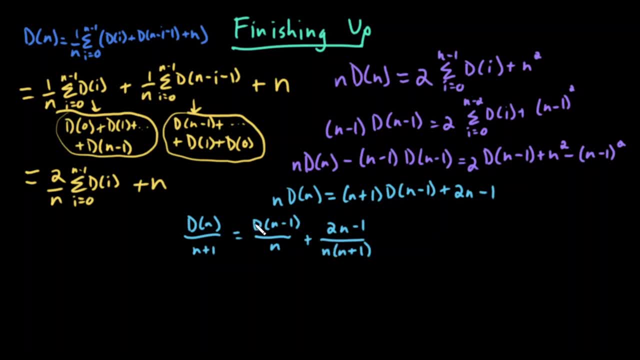 And once we, if we basically do, n equals 1, so if we have n equals 1, the base case would be d of 1.. So d of 1 equals n over 2, equals d of 0 over 1 plus 2 minus 1 over 1 times 2.. 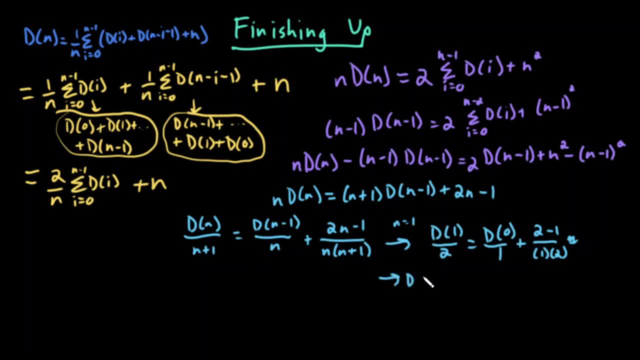 So basically, d of 1 equals 1, because, oh actually so d of 0.. what is D of zero? D of zero is the expected total depth of a tree that has zero nodes. That's, by definition, zero. Therefore, D of one is one. And then 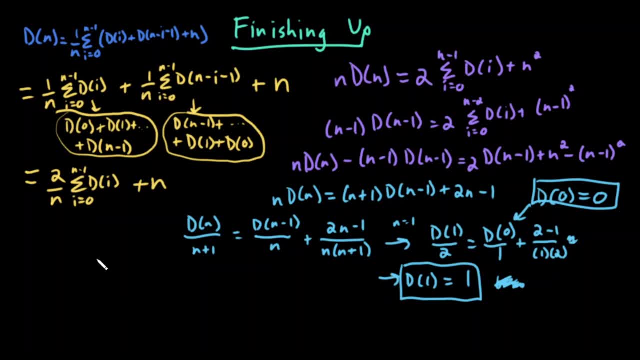 collecting my terms, I would get- let me use a different color for this now- I would get: D of n over n plus one equals the sum from i equals one to n of two. i minus one over i times quantity. i plus one, which is the sum from i equals one. 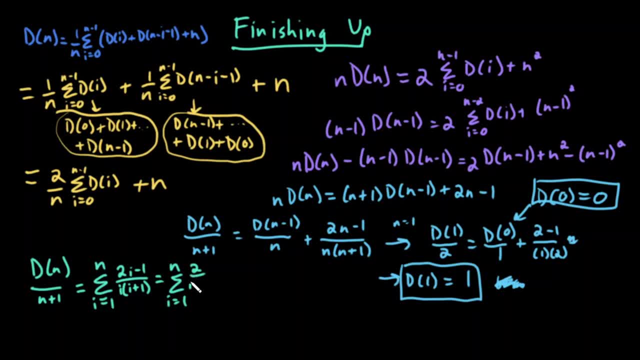 to n of two over i plus one. minus, the sum from i equals one to n of one over i times i plus one, And I can further simplify this using induction. I won't show it here, but I'll just summarize. So: the sum from i equals one to n of one over i times. 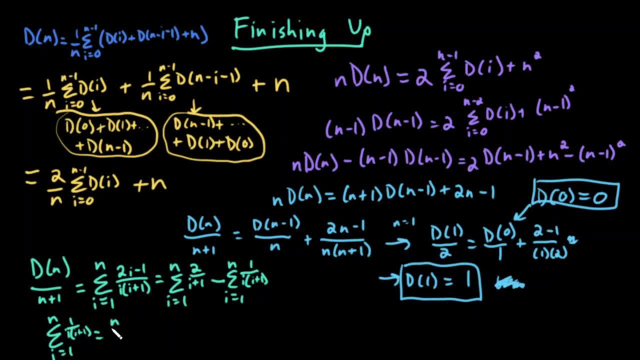 this is i plus one minus. the sum from i equals one to n of two over i plus one. i times i plus one equals n over n plus one. So therefore a lot of parts. but therefore we get: sum from i equals one to n of two over. i plus one equals two times the sum from i. 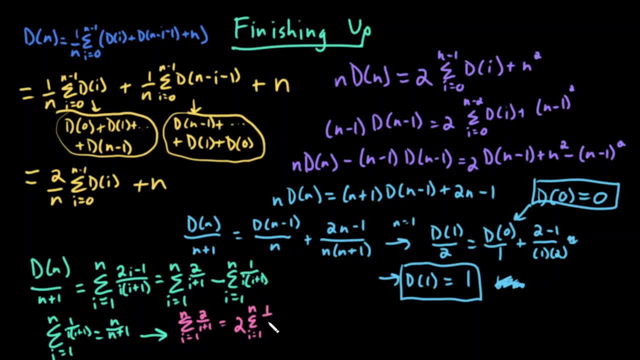 equals one to n of two over i plus one. So therefore we 얘 l�100.. Is the right fully n of 1 over i plus 2 over n plus 1 minus 2, which equals 2 times the sum from i. equals 1 to n of 1 over i, minus 2n over n plus 1. so the closed form solution to. 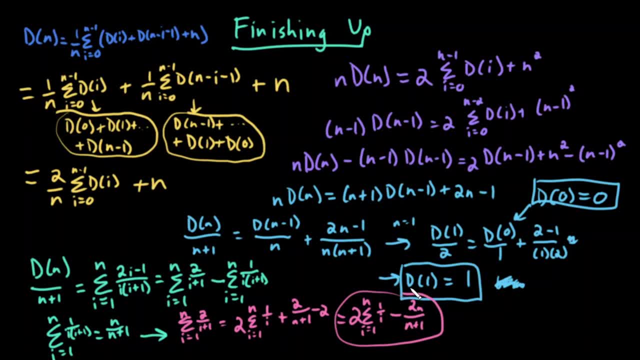 this. so this is finally getting to the end. the closed form solution here: d of n equals d of n equals 2n plus 1 times the sum of i equals 1 to n of 1 over i minus 3n. if you didn't. 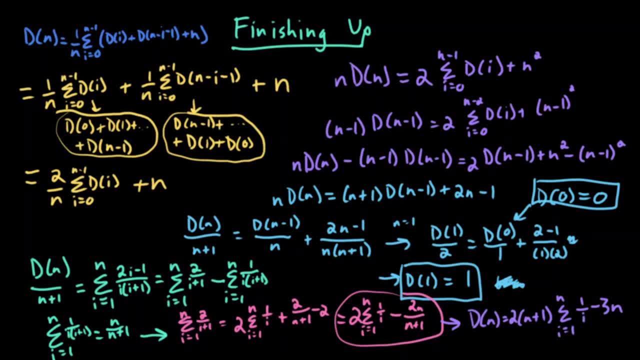 fully follow what just happened, don't worry about it. uh, the math is a little complex, but it's not essential to totally follow. uh, basically the last step. this is the last last step. i promise we can approximate this as d of n is basically so this is very similar. 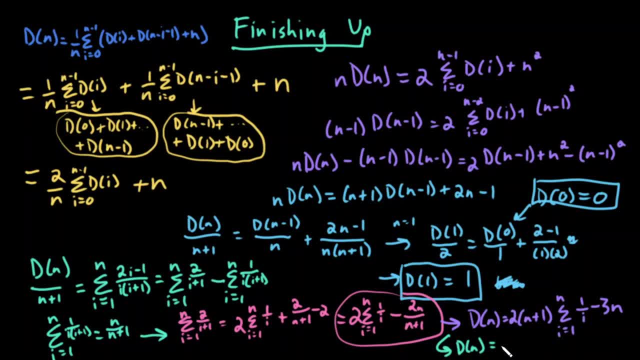 to well actually, so i'll just- i don't think i'll do the last step- so we can approximate this to basically show that the expected value of a find operation is roughly 2 times quantity n plus 1 over n times natural log of n minus 3. how i got this? don't worry about it. uh, there's an approximation. 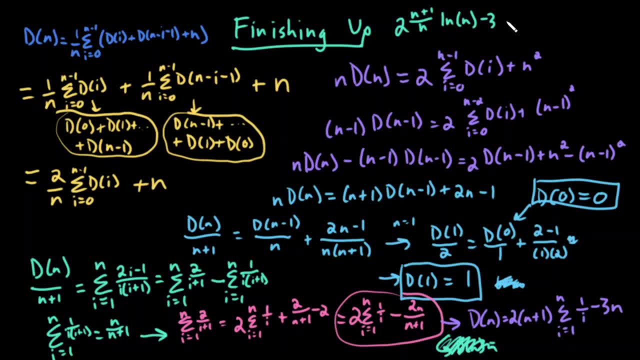 that i made to get here, which is approximately 1.386 times log base 2 of n 3. all that matters to you. so if you didn't follow anything in this super, super, super lengthy derivation, all that matters is this log base 2 of n term. it's some constant times log base 2 of n. 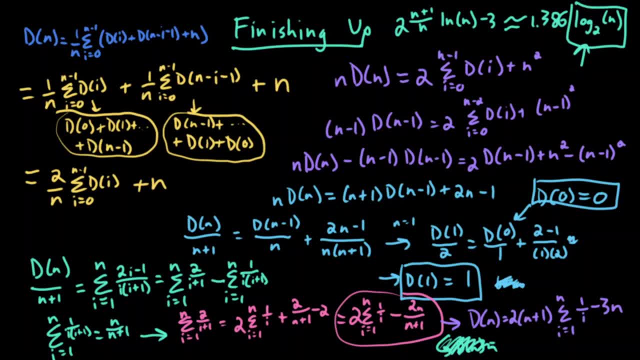 so all we care about is that this shows that this is in expectation. big o of log n. 3, 4, 5, 6, 7, 8. We did it, So don't worry about the math If it didn't make all the world all the best sense. 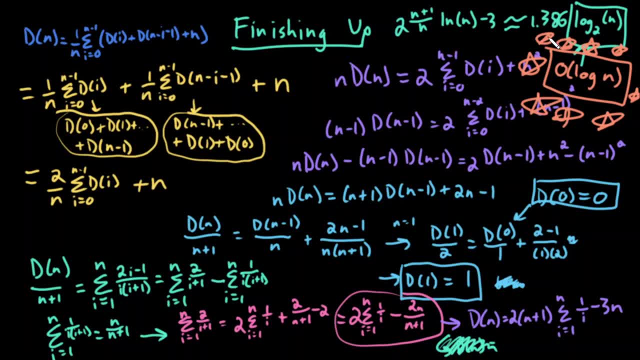 The basic takeaway of this entire super, super, super lengthy mathematical derivation is that we have shown that, given those two assumptions we made at the beginning, that the big O average case time complexity of doing a find operation is indeed big O of log n, 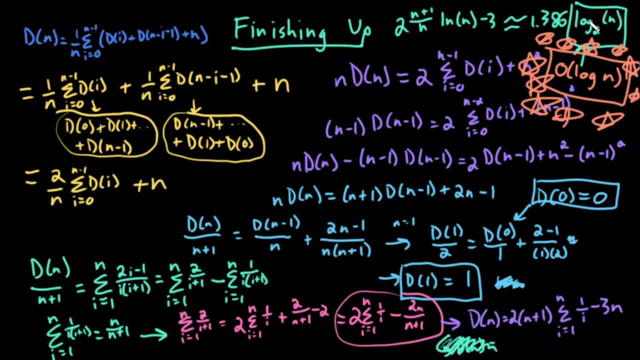 It's approximately 1.386 times log of these two of n. but all we care about in big O is that it's big O of log n, Some retrospect. So we made two assumptions. We assumed that all insertion orders are equally likely. 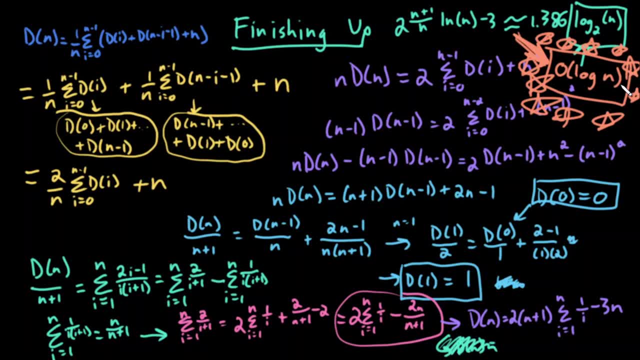 and we assumed that we will be equally likely searching for any given element in our tree. These two assumptions are not the most realistic with real data. So under these simplifying assumptions we get an expected value of big O of log n. but this doesn't necessarily hold with real world data. 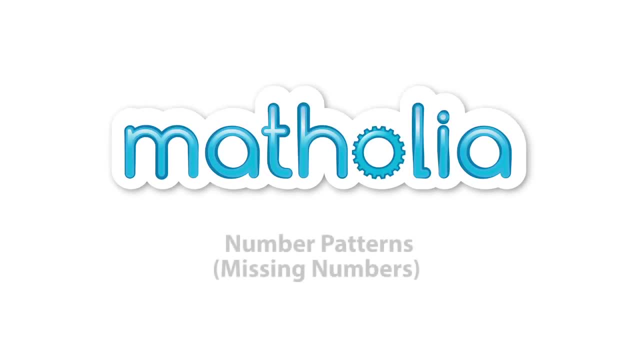 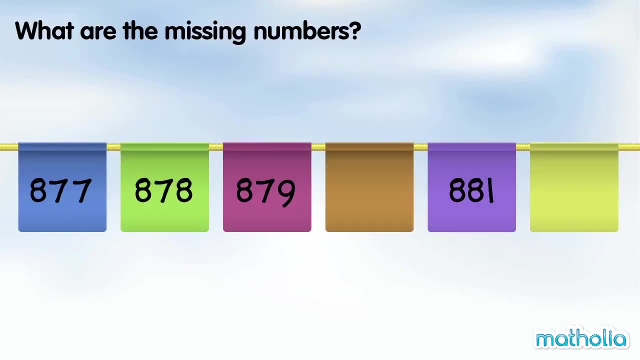 What are the missing numbers? 877 plus 1 is 878.. 878 plus 1 is 879.. In each step the numbers go up by 1.. 879 plus 1 is 880.. 881 plus 1 is 882.. 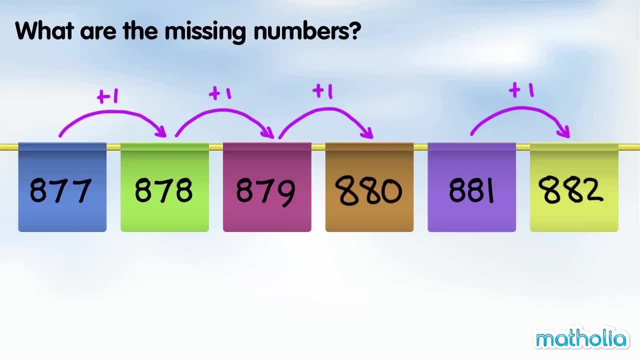 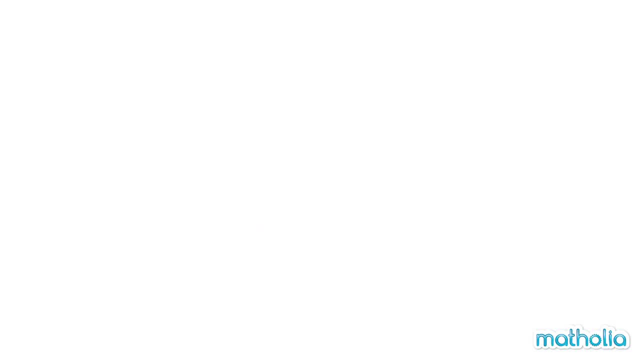 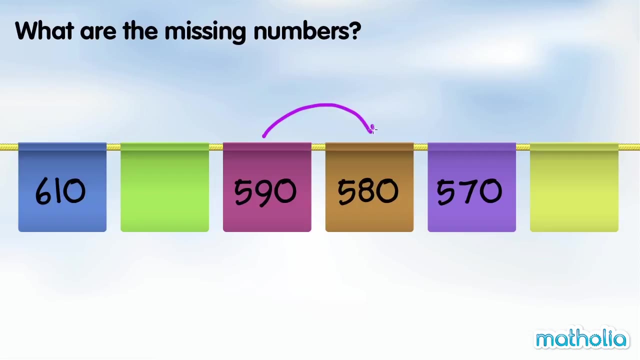 The missing numbers are 880 and 882.. What are the missing numbers? 590 minus 10 is 580.. 580 minus 10 is 570.. In each step the numbers go down by 10.. 610.. Minus 10 is 600.. 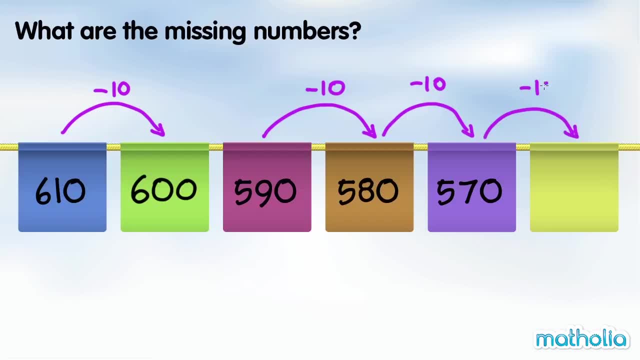 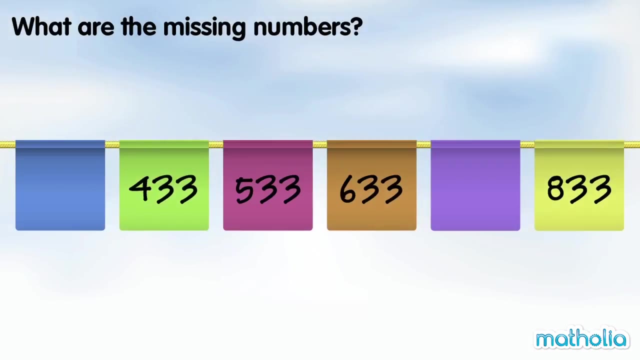 570 minus 10 is 560.. The missing numbers are 600 and 560.. What are the missing numbers? 433 plus 100 is 533.. 533 plus 100 is 633.. In each step the numbers go up by 100..